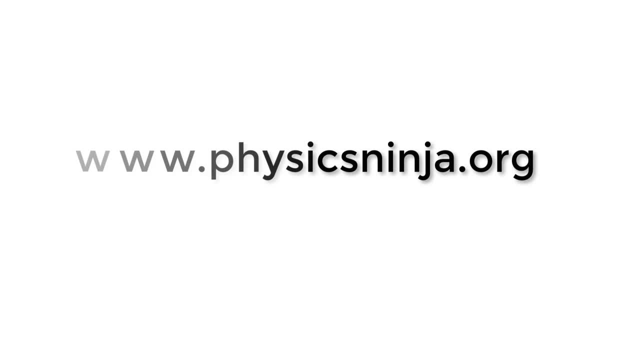 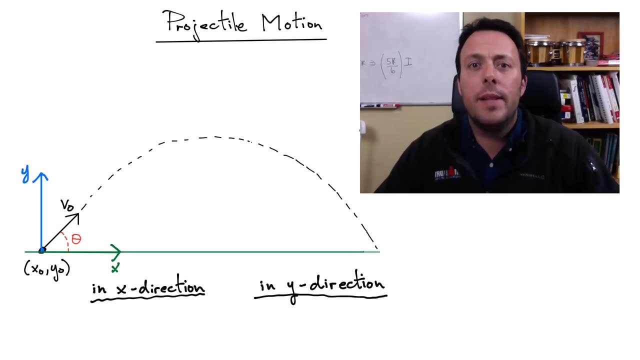 Hi, today I want to talk about projectile motion. So here's the setup: I'm assuming that I'm launching a projectile at some angle with respect to the horizontal and the angle is theta. I'm launching the object at some initial velocity v0, and I want to look at the motion. 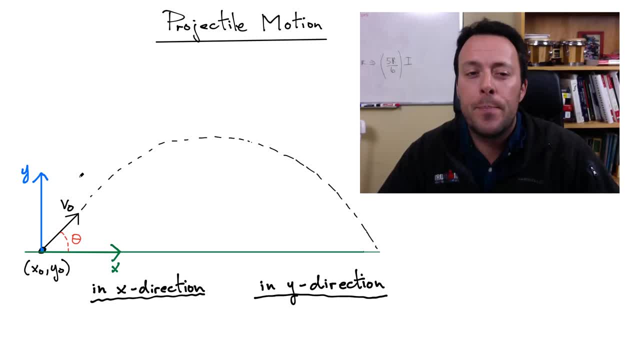 of this particle as it travels through the air. So the first thing we want to do is define a coordinate system. So I've done that here, So I'm going to call everything pointing up that'll be in the positive y direction and everything pointing to the right is going. 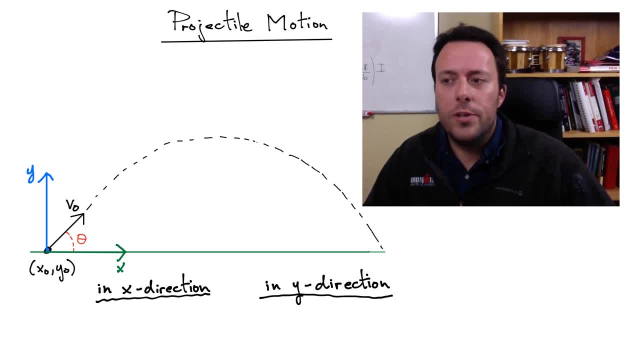 to be in the positive x direction. So when describing the projectile through the air, the key thing to remember in this is that things that are happening in the x direction are kind of independent from what's going on in the y direction. So we're analyzing. 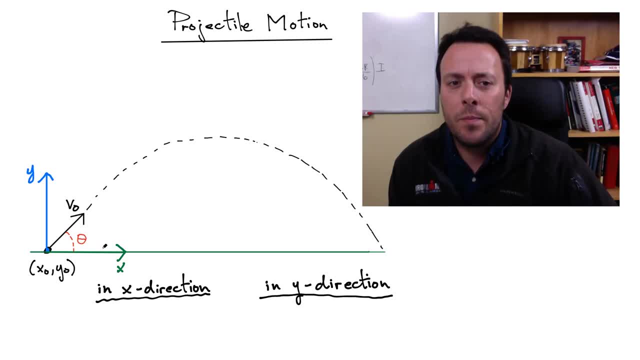 the motion along each direction kind of independently. They're linked together by time, but still we want to break things down and look at each component separately. So the first thing we're going to do is we're going to break the initial velocity down into two components. So let me redraw this initial velocity, that's at 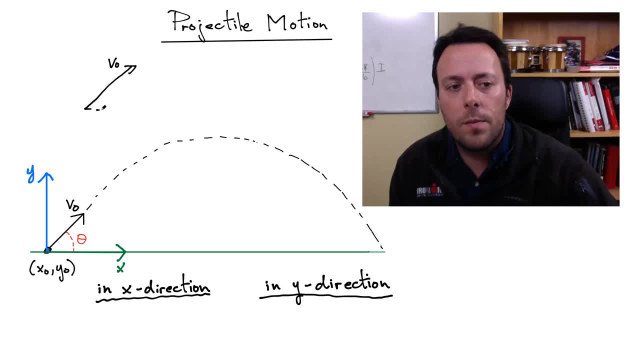 some angle. The magnitude of the vector is v0, and our angle was theta, and that was defined with respect to the horizontal. So the first thing I want to do is I want to break that down into two components. So, again, my coordinate system is defined by this x axis and the y axis. so I want to break. 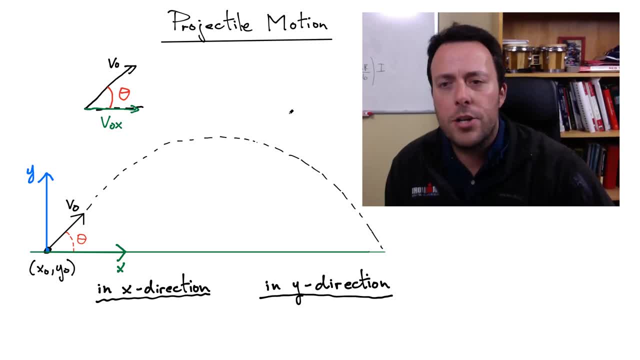 things down into an initial velocity in the x direction and also some initial velocity in the y direction. Now, just by inspection, you should be able to write that the initial component of the velocity in the x direction is going to be v0.. 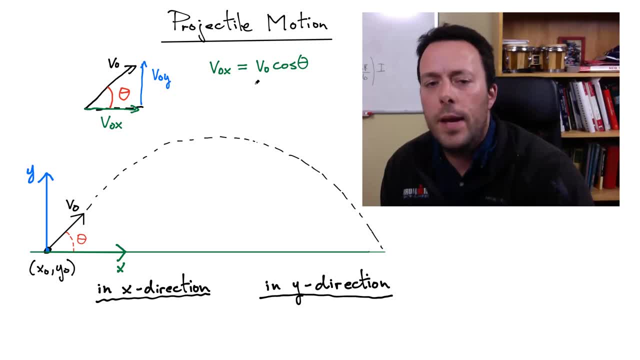 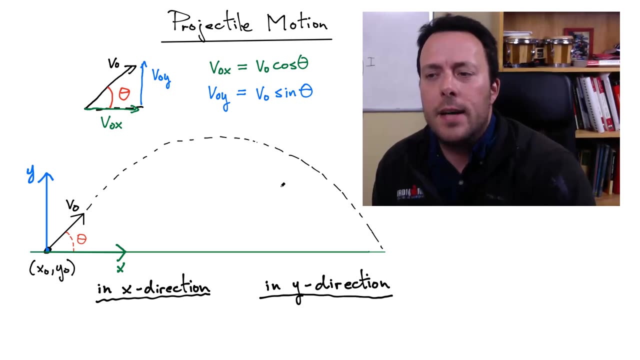 Cos of the angle theta, And the initial component of the velocity in the y direction is going to be v0, sine of the angle theta. Alright, now the next thing I want to do is I also want to write what is the direction of the acceleration everywhere in space. 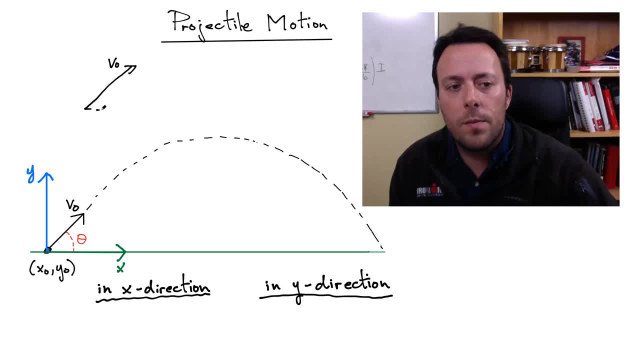 some angle. The magnitude of the vector is v0, and our angle was theta, and that was defined with respect to the horizontal. So the first thing I want to do is I want to break that down into two components. So, again, my coordinate system is defined by this x axis and the y axis. so I want to break. 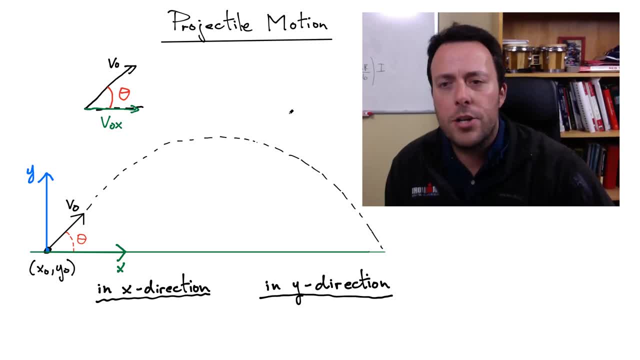 things down into an initial velocity in the x direction and also some initial velocity in the y direction. Now, just by inspection, you should be able to write that the initial component of the velocity in the x direction is going to be v0.. 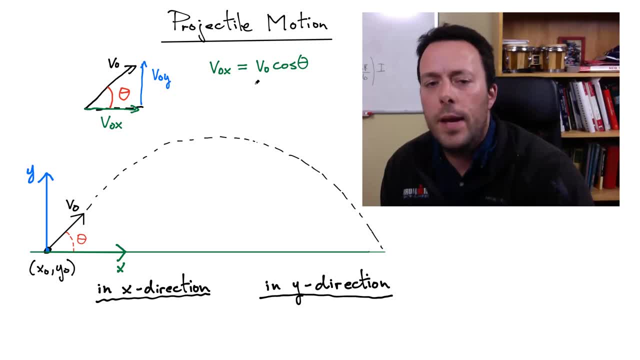 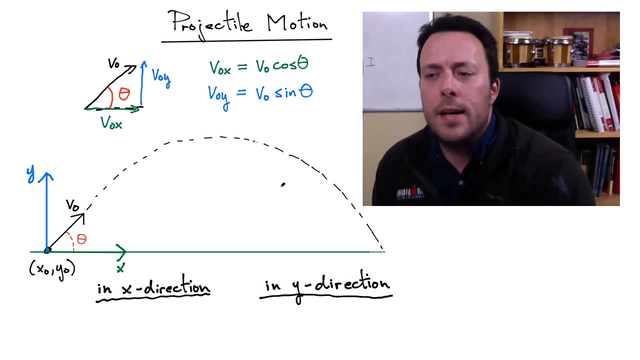 Coase of the angle theta, And the initial component of the velocity in the y direction is going to be v0, sine of the angle theta. Alright, Now the next thing I want to do is I also want to write what is the direction of the acceleration everywhere in space. 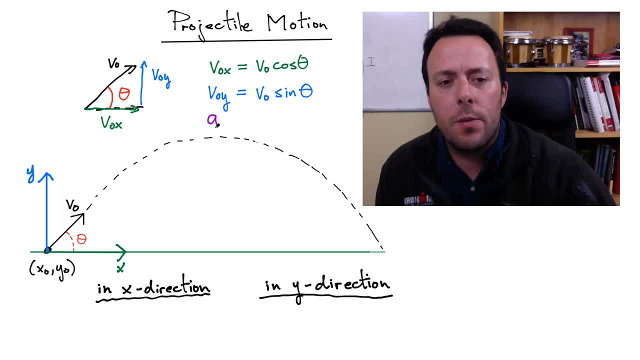 Now you have to be a little bit careful with this. So I want to write the acceleration And, if you remember, this is a case of uniform acceleration, So you could typically use a uniform acceleration, But the speed in your generalно-level Johannessens can be 100% opposite one. In HERE you can use a. 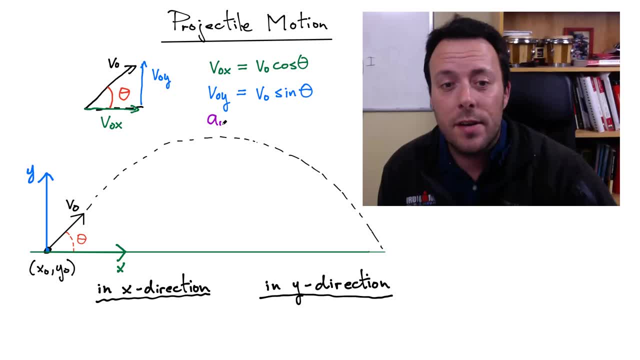 acceleration. So the acceleration is constant. It's always going to be in the y-direction and if I plot it anywhere on this dashed line which represents the trajectory of my projectile, the acceleration is always going to point down. If I plot it near the top, the acceleration is pointing down. If I plot 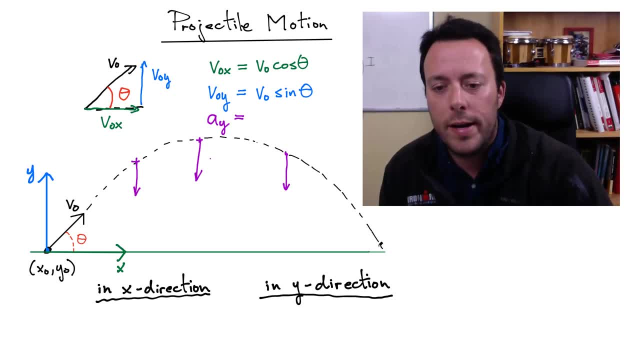 it near the second half of the trajectory. it's also pointing down If I plot the acceleration right before it hits the ground. it's also pointing down The magnitude now is going to be little g, and it's little g everywhere and again our little g will be. the magnitude will be 9.8. 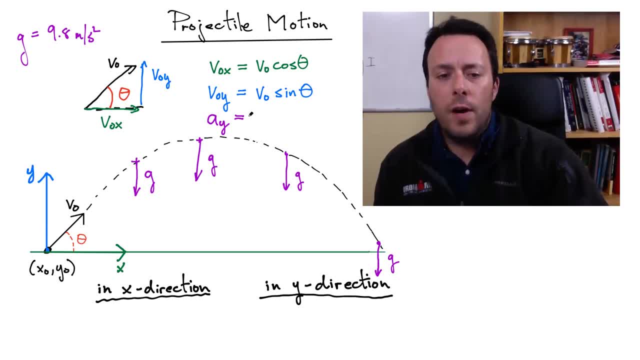 meters per second squared. So if I want to write the acceleration now, I really have to write it with respect to a coordinate system. You know it's pointing down. so if it's pointing down- and it's- it has a magnitude of 9.8.. The way you write that now is going to be. it's going to be. 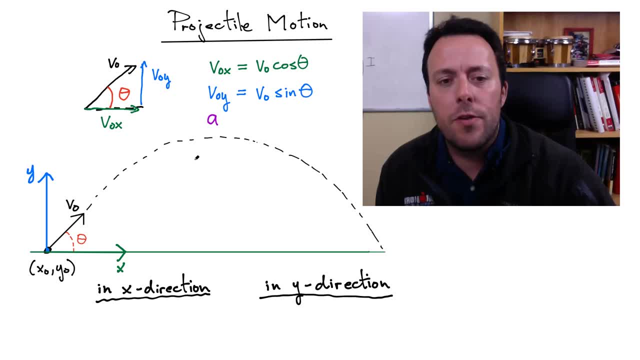 Now you have to be a little bit careful with this. So I want to write the acceleration And, if you remember, this is a case of uniform acceleration acceleration. So the acceleration is constant. It's always going to be in the Y direction. 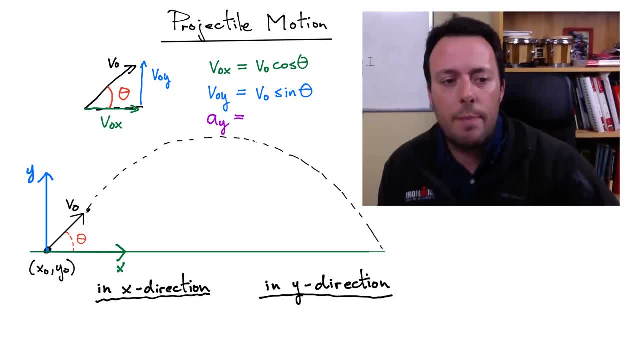 And if I plot it anywhere on this dashed line which represents the trajectory of my projectile, the acceleration is always going to point down. If I plot it near the top, the acceleration is pointing down. If I plot it near the second half of the trajectory, it's also pointing down. 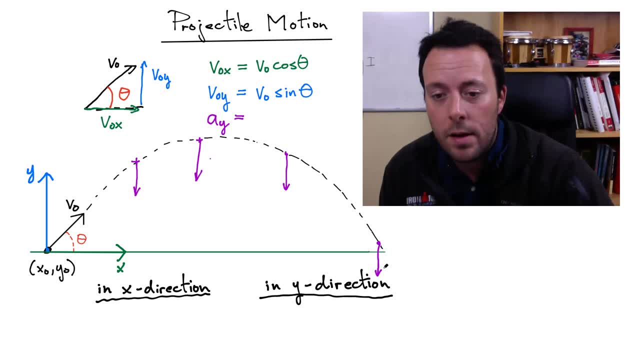 If I plot the acceleration right before it hits the ground, it's also pointing down The magnitude. now is going to be little g, And it's little g everywhere, And again our little g will be the magnitude will be 9.8 meters per second squared. So if I want to write the acceleration now, 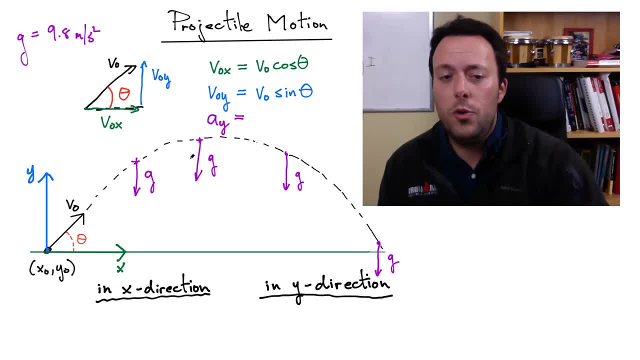 I really have to write it. with respect to a coordinate system. You know it's pointing down. So if it's pointing down, it's pointing down. So if it's pointing down, it's pointing down. So if it's pointing down, it's pointing down. 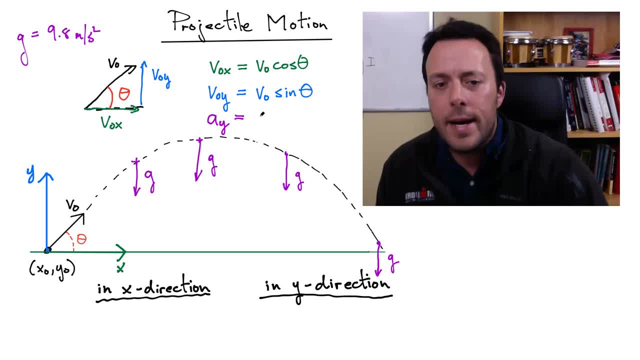 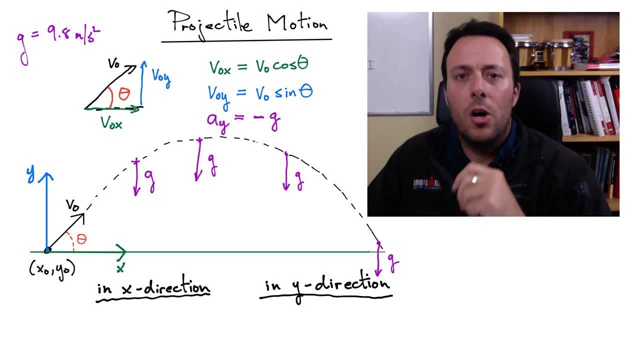 If it's pointing down and it has a magnitude of 9.8, the way you write that now is going to be: it's going to be equal to minus little g. Okay, we're now in a position to analyze the motion, because we know the initial velocity. 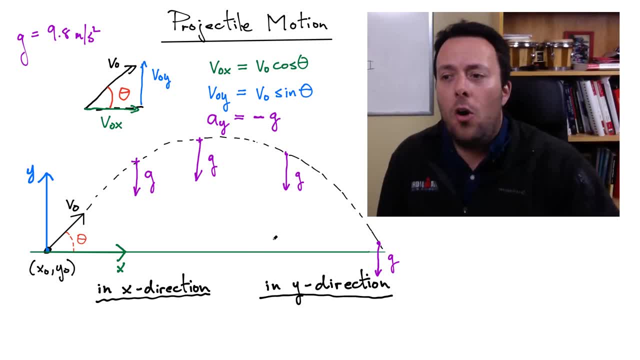 and I know the acceleration at every point in time. All I want to do now is I want to write expressions that are going to tell me the X direction displacement and the velocity, and also the displacement in the Y direction and the velocity in the Y direction as a function of time. 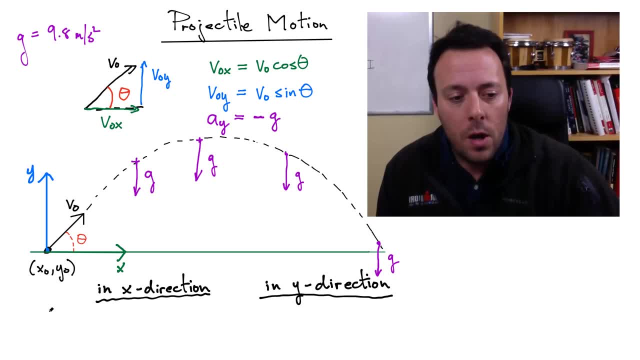 So let's start with the displacement in the X direction. So I'm going to write it as X minus X0.. So I'm starting from some initial position here and let's just call this delta X. That is the displacement from the origin. 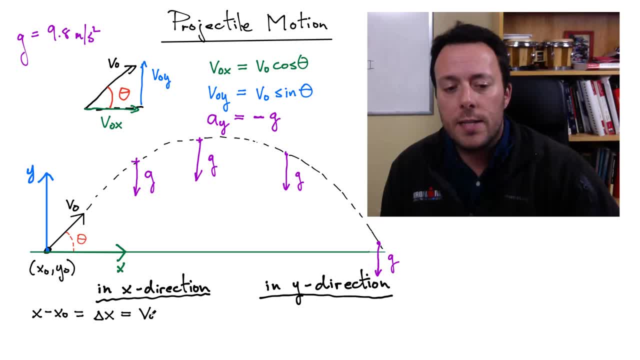 So this here is simply equal to the initial velocity in the X direction multiplied by time. Now there's no other term for the X displacement, because there is no acceleration in the X direction, The acceleration is only pointing down, That's in the Y direction. 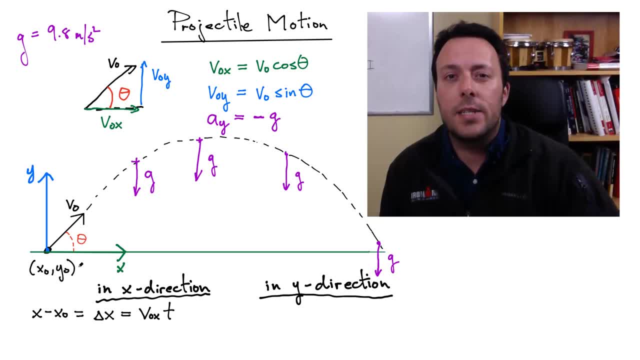 The next thing we want to do now is also describe the velocity in the X direction. So, in order to do that simply, the velocity in the X direction is going to be equal to the initial velocity in the X direction, and well, that's it. 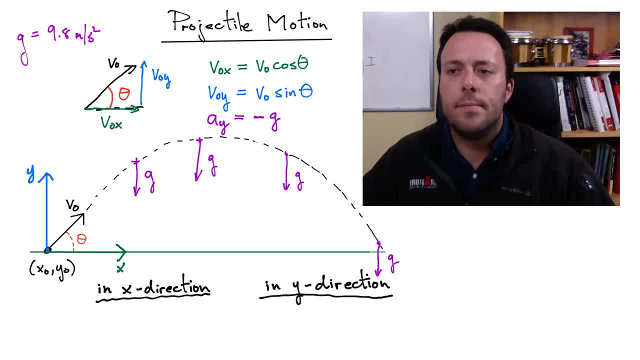 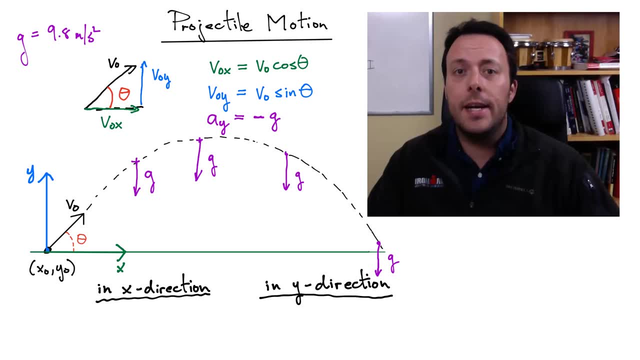 equal to minus little g. Okay, we're now in a position to analyze the motion, because we know the initial velocity and I know the acceleration at every point in time. All I want to do now is I want to write expressions that are going to tell me the x direction, displacement and 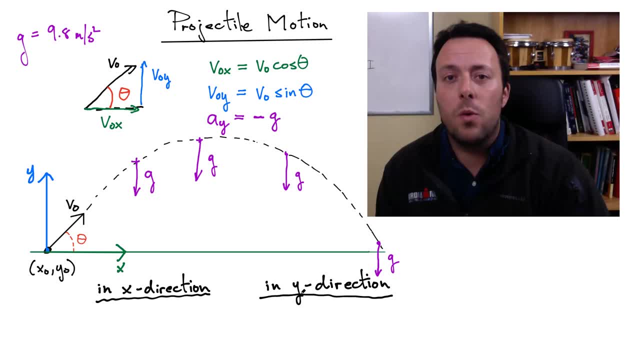 the velocity and also the displacement in the y direction and the velocity in the y direction as a function of time. So let's start with the displacement in the x direction. So I'm going to write it as x minus x0.. So I'm starting from some initial position here. 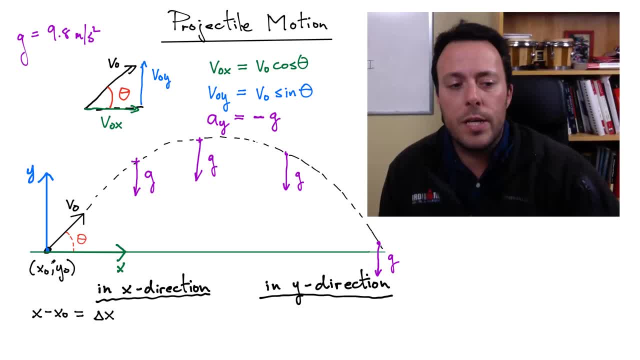 and let's just call this delta x. That is the displacement from the origin. So this here is simply equal to the initial velocity in the x direction multiplied by time. Now there's no other term for the x displacement, because there's no acceleration in the x direction. 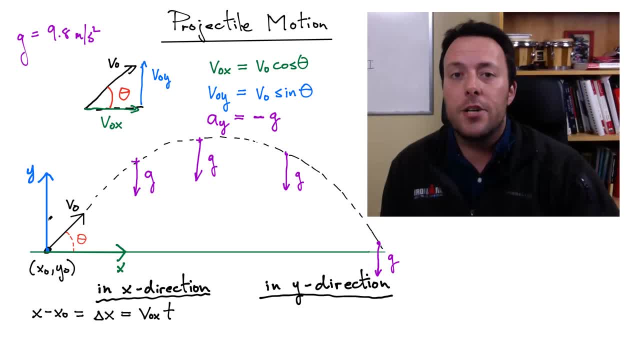 The acceleration is only pointing down, That's in the y direction. The next thing we want to do now is also describe the velocity in the x direction. So, in order to do that simply, the velocity in the x direction is going to be equal to the initial velocity in the x. 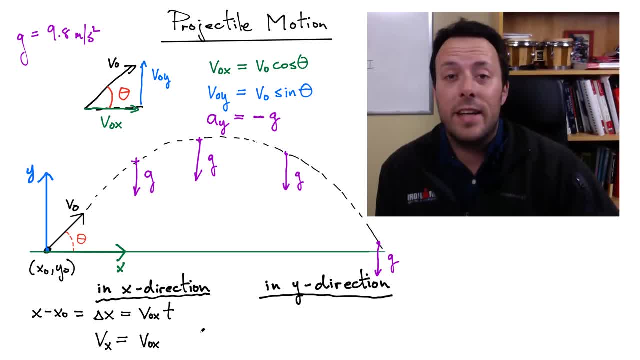 direction. and well, that's it. There's nothing else to add. The equations of motion in the x direction are very, very easy to write, because there's no acceleration in the x direction. So let's repeat the same exercise now for the y direction. It's a little bit more complicated. 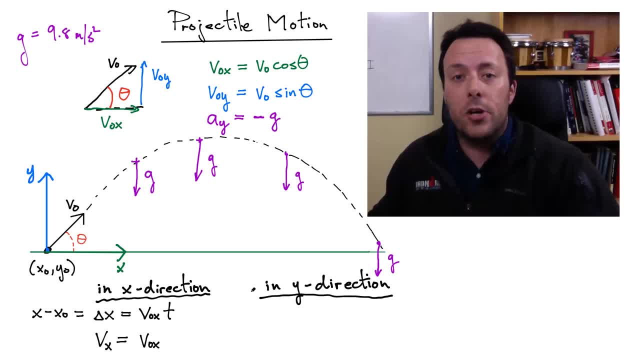 in the y direction because there's acceleration, So we need to add a term that describes its effects. So the displacement in the y direction, which is y minus my initial position where I started, is going to be equal to delta y. And now, well, 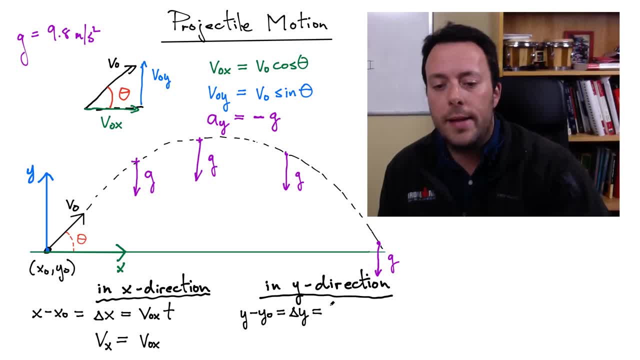 in the y direction, the first term looks similar to what we had in the x, except we have to plug in the initial velocity in the y direction multiplied by time, And now there's a term with acceleration And if I factor in the sine, which is negative for this case because 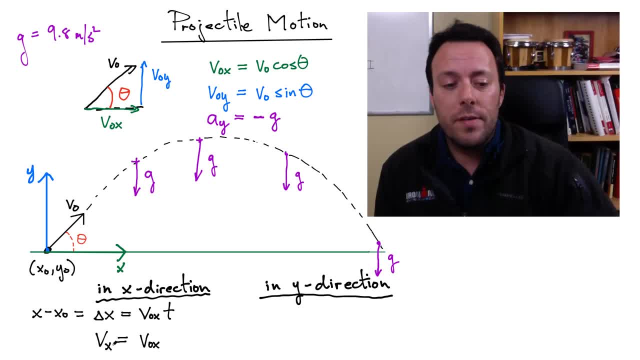 There's nothing else to add. The equations of motion in the X directions are very, very easy to write because there's no, there's no acceleration in the X direction. So let's repeat the same exercise now for the Y direction. It's a little bit more complicated in the Y direction because there's acceleration. 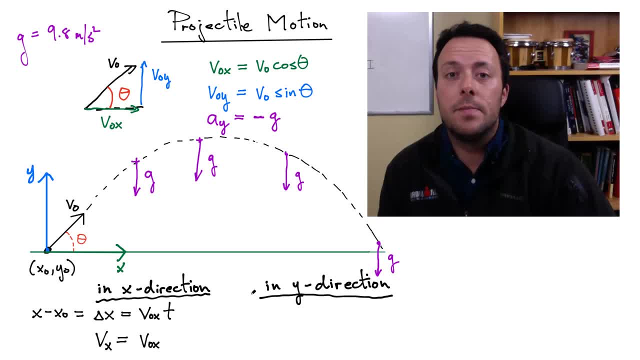 So we need to add a term that describes its effects. So the displacement in the Y direction, which is Y minus my initial position where I started, is going to be equal to delta Y. And now, well, the displacement in the Y direction. 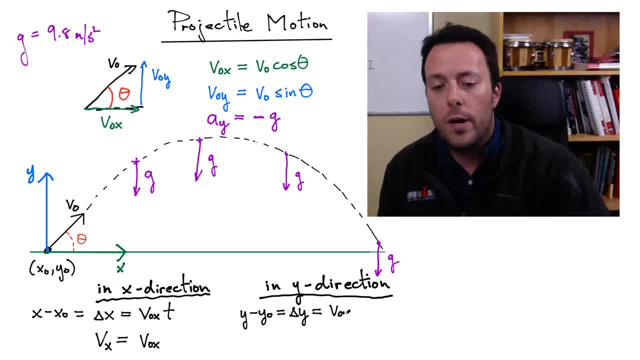 the first term looks similar to what we had in the X direction. It's going to be equal to delta X, except we have to plug in the initial velocity in the Y direction multiplied by time, And now there's a term with acceleration. 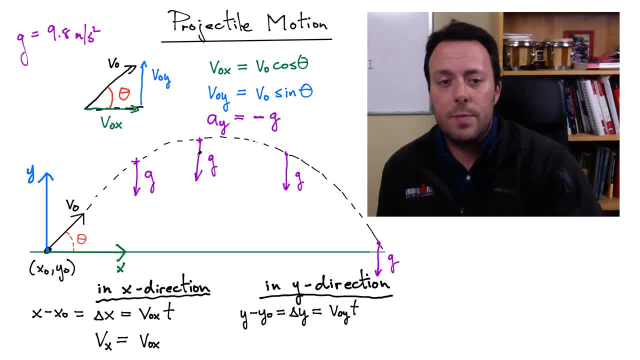 And if I factor in the sign, which is negative for this case because the acceleration is down, this term will simply become one-half negative, one-half G T squared, And the negative reflects the fact that my acceleration is minus G Again. this is just the simple kinematic equation. 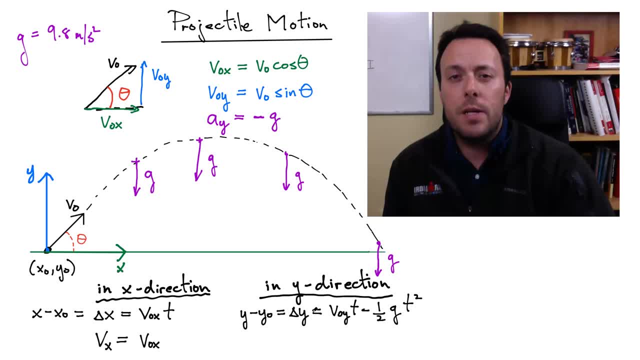 It gives you the displacement of an object that has constant acceleration. The last thing I need to do now is I need to tell you what is the vertical component of the velocity as a function of time. That's going to be equal to my initial component of the velocity. 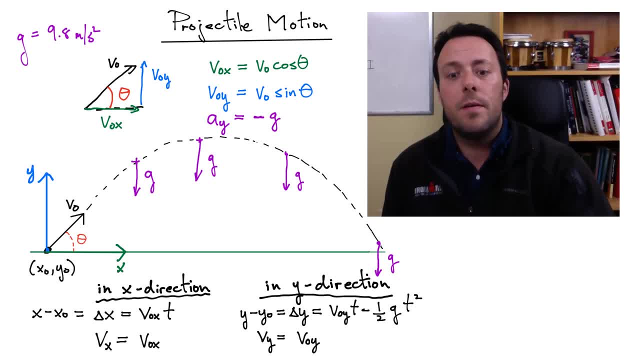 which is V naught sine theta that I have up above. And now there's also a term that describes the acceleration And that will be minus the acceleration times the velocity. That's going to be minus the acceleration times the velocity. So there you have it. 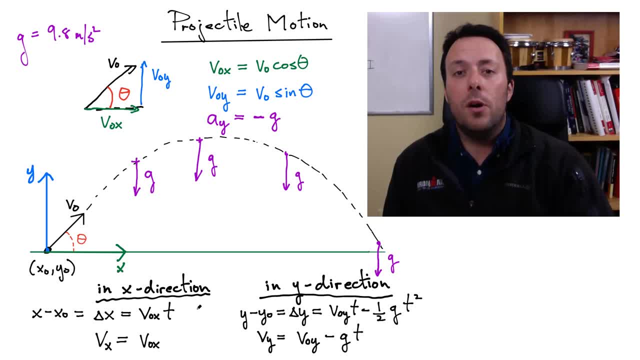 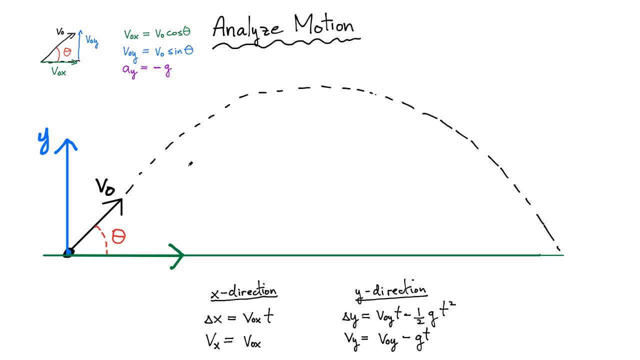 We have equations that give us the displacements in both the X and the Y direction, And we also have equations that give us the velocity in the X and the Y direction. Okay, so I want to first analyze the motion, at least qualitatively. 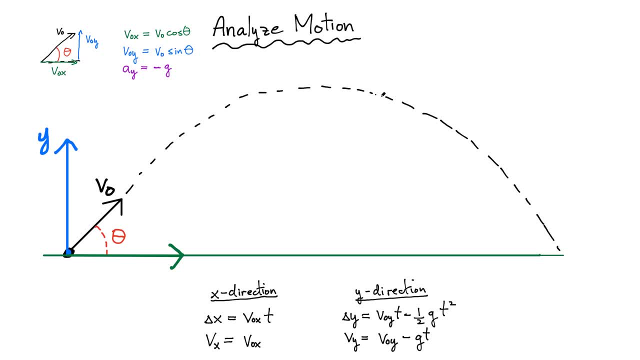 So let's first examine what's going on to the velocity as the projectile moves along this path. One thing we notice is: let's plot the magnitude of this initial velocity in the X direction. So we have a vector that's about this long and that is the initial velocity in the X direction. 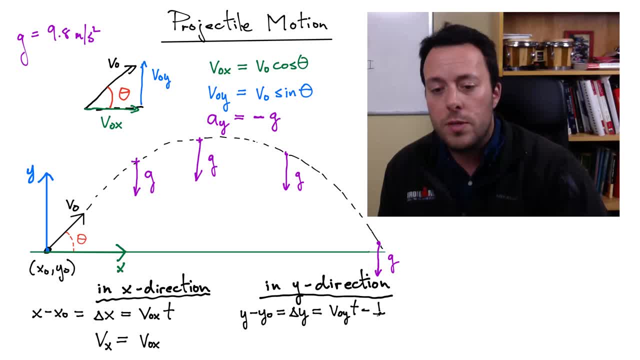 the acceleration is down. this term will simply become one-half negative, one-half gt squared, And the negative reflects the fact that my acceleration is minus g Again. this is just the simple kinematic equation that gives you the displacement of an object that has constant. 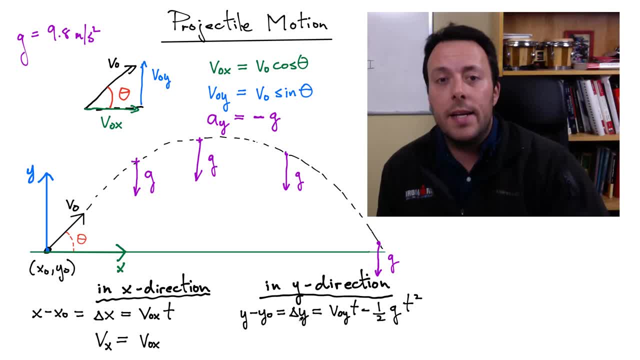 acceleration. The last thing I need to do now is I need to tell you what is the vertical component of the velocity as a function of time, That's going to be equal to my initial component of the velocity, which is v, naught sine theta that I have up above, And now there's. 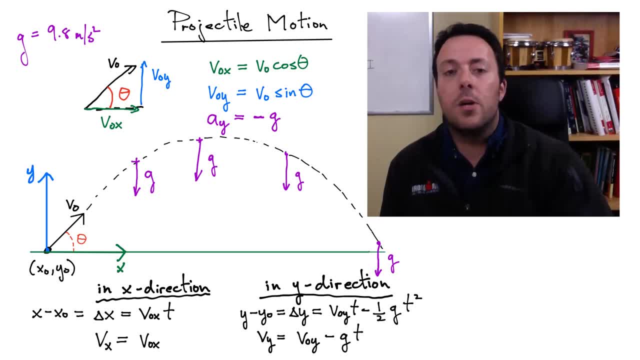 also a term that describes the acceleration, and that will be minus the acceleration times time. So there you have it. We have equations that give us the displacements in both the x and the y direction, and we also have equations that give us the velocity in the x and the y direction. 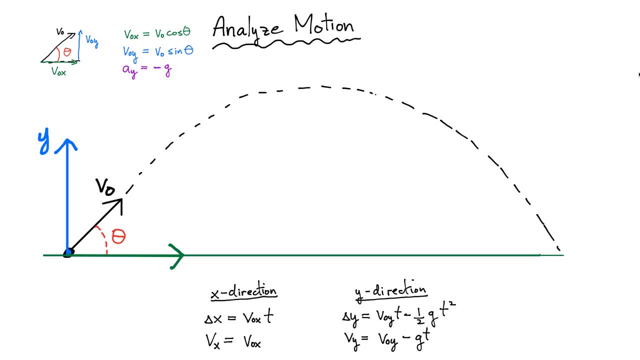 Okay. so I want to first analyze the motion, at least qualitatively. So let's first examine what's going on to the velocity as the projectile moves along this path. One thing we notice is: let's plot the magnitude of this initial velocity in the x direction. We have a vector. 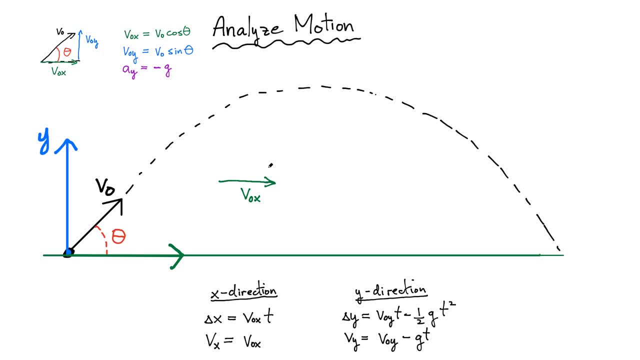 that's about this long and that is the velocity in the x direction. So let me cut and paste at different points along this trajectory. Well, what if we're over here at this point? That's the initial velocity. And you notice, if I look at my equation of motion down here. 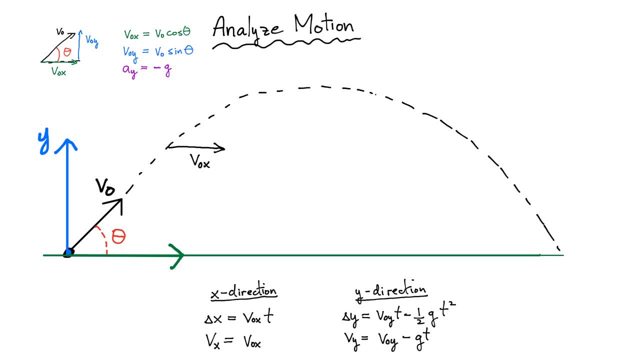 that gives me the x velocity versus time. one thing I notice is that for every single time- this is my equation- It doesn't change. So what does that mean? That means that this vector over here is always going to be the same length If I plot it over at this position. 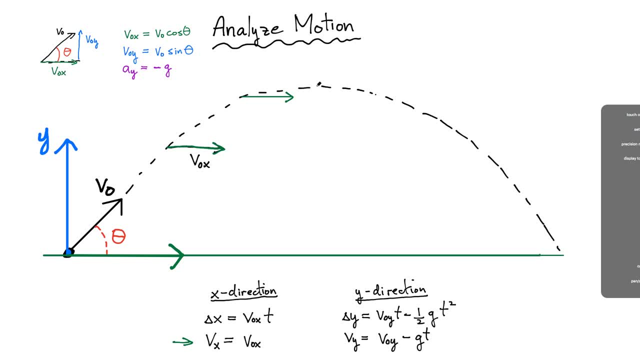 I get a vector that's roughly the same length. It's the same length. rather, If I plot it at the top, I'm going to get a vector that's the same length. So the velocity at every single point, at least in the x direction, is always the same, Even down over here it's. 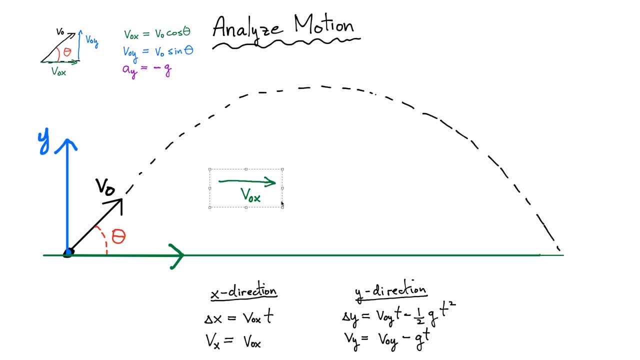 So let me cut and paste this And let's place it at different points along this trajectory. Well, what if we're over here at this point? That's the initial velocity And you notice, if I look at my equation of motion down here. 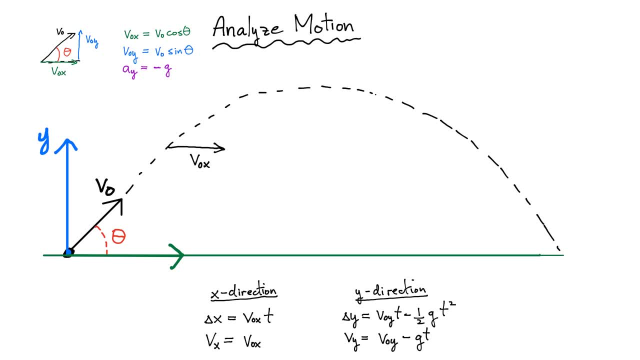 that gives me the X velocity versus time. what I notice is that for every single time- this is my equation, It doesn't change. So what does that mean? That means that this vector over here is always going to be the same length. 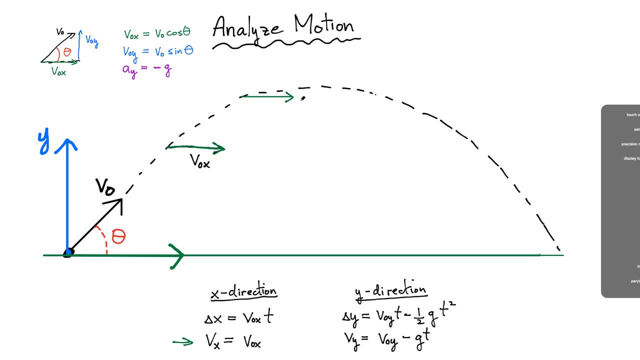 If I plot it over at this position, I get a vector that's roughly the same length. It's the same length. rather, If I plot it at the top, I'm going to get a vector that's the same length. So the velocity at every single point. 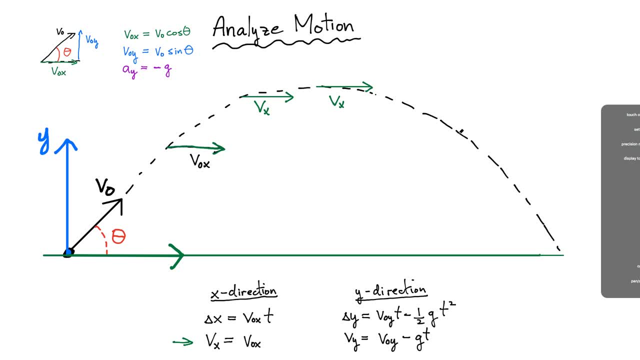 at least in the X direction, is always the same, Even down over here. It's a vector that's the same length Right as it hits the ground The instant before it hits the ground. That's the magnitude of my velocity in the X direction. 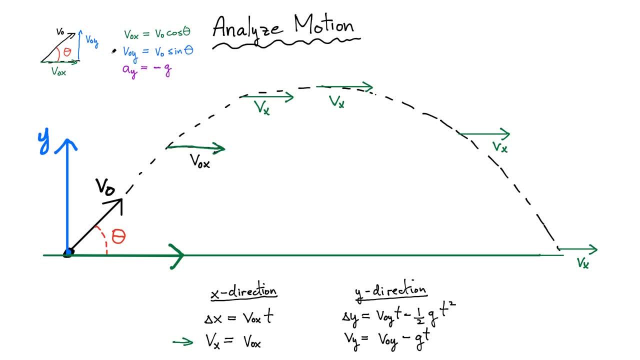 Now let's look at what's going on in the Y direction. In the Y direction, initially, I have a vector that's pointing up, So I can go ahead and plot it right here. This is my initial velocity in the Y direction. It's this vector here. 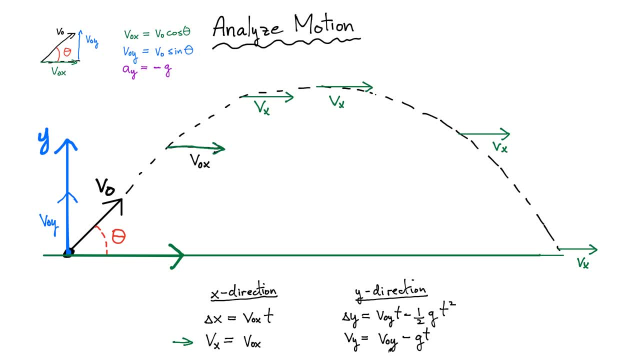 Okay, And let's look at what happens as a function of time. Well, again, if you look at my expression now for the velocity as a function of time, I have an initial term and now I'm subtracting a little bit of. 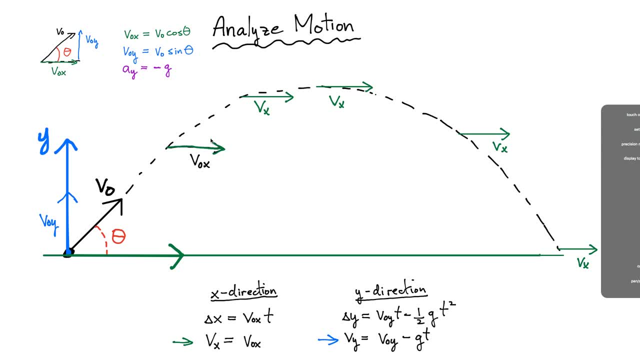 I'm subtracting another term here. So what does that mean? That means it's getting smaller. So my velocity in the Y direction is a vector. now that is getting slightly smaller as time goes on, As I near the top. let's have a look at that vector. 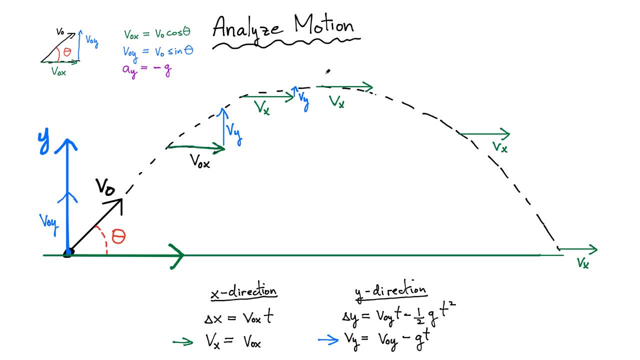 It's very, very small. And once I'm right at the top, I can't actually even plot it, because the component of the velocity in the Y direction equals to zero at the top. And then what happens- Look at this expression- After time gets beyond a certain value. 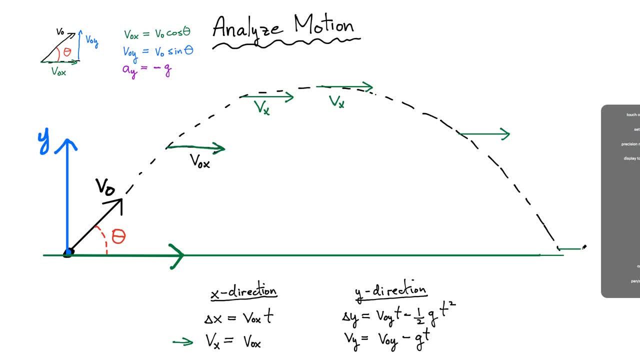 a vector that's the same length Right as it hits the ground the instant before it hits the ground. that's the magnitude of my velocity in the x direction. Now let's look at what's going on in the y direction. In the y direction, initially, I have a vector. 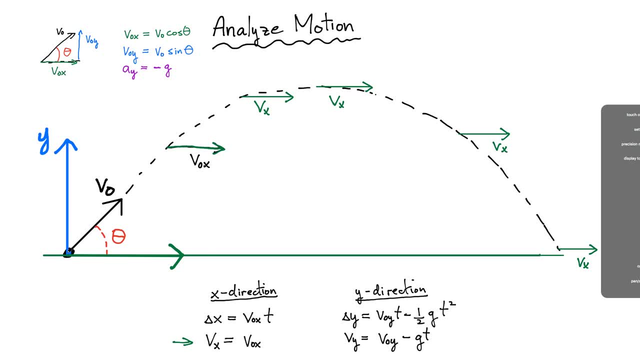 that's pointing up, So I can go ahead and plot it right here. This is my initial velocity in the y direction. It's this vector here. Okay, and let's look at what happens as a function of time. Well, again, if you look at my expression now for the velocity as a function of time, I have 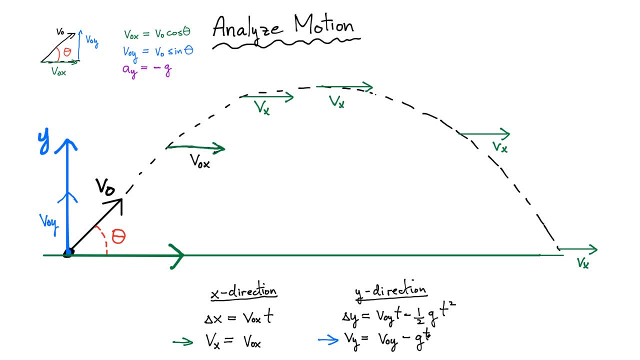 an initial term and now I'm subtracting a little bit of, I'm subtracting another term here. So what does that mean? That means it's getting smaller. So my velocity in the y direction is a vector now. that is getting slightly smaller as time goes on. 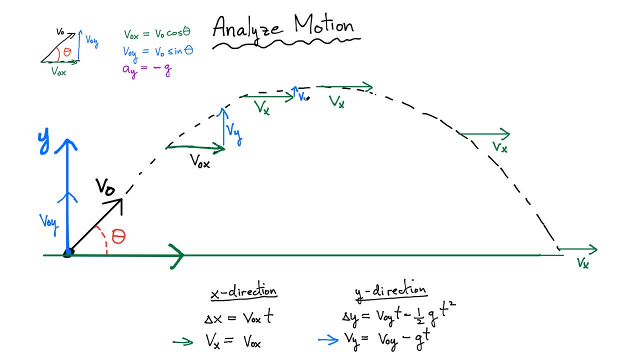 As I near the top. let's have a look at that vector. It's very, very small and once I'm right at the top, I can't actually even plot it, because the component of the velocity in the y direction equals to zero at the top. And then what happens? Look at this expression. 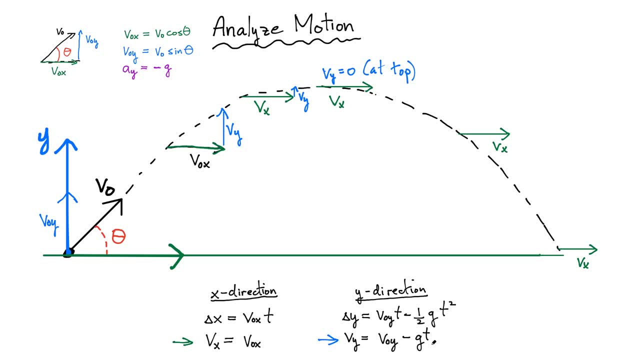 After time gets beyond a certain value, the second term here is going to be bigger than my initial velocity term. So the term that has a certain value is going to be bigger than my initial velocity term. So the term that has a certain value is going to be bigger than my initial velocity term. 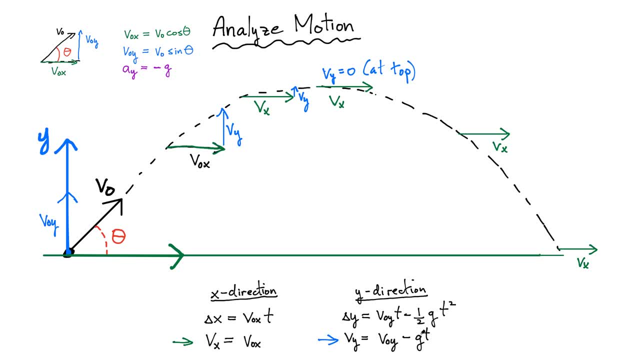 So that's going to mean that the velocity in the y direction, as the gravity multiplied by the time, will become bigger, And that means overall, the velocity in the y direction will become negative. And for a vector to become negative, that basically means that 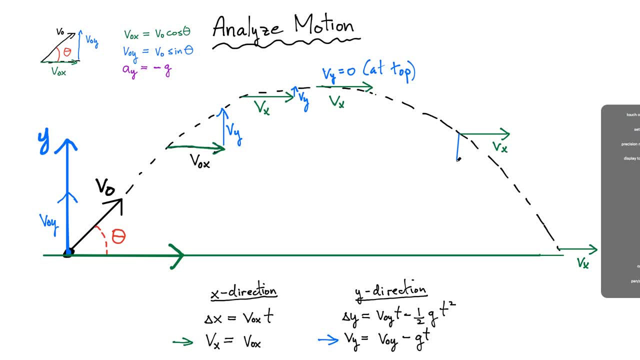 I'm simply changing directions. So after a certain amount of time this is what's happening. So the velocity in the y direction basically just switches sign and then becomes bigger at the time. So it'll look something like that At every single point in time. now, since I know the magnitudes of each component, I can go ahead and plot the vector Vy as a function of time. 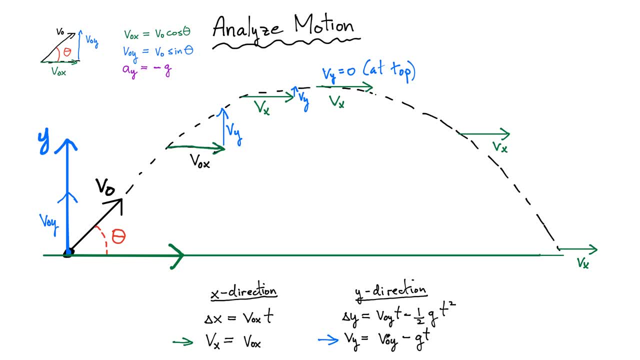 the second term here is going to be bigger than my initial velocity term. So the term that has the gravity multiplied by the time will become bigger and that means overall the velocity in the Y direction will become negative And for a vector to become negative 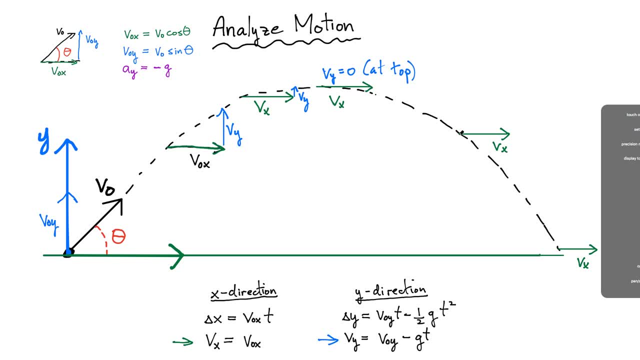 that basically means that I'm simply changing directions. So after a certain amount of time, this is what's happening. So the velocity in the Y direction basically just switches, sign and then becomes bigger with time. So it'll look something like that At every single point in time now. 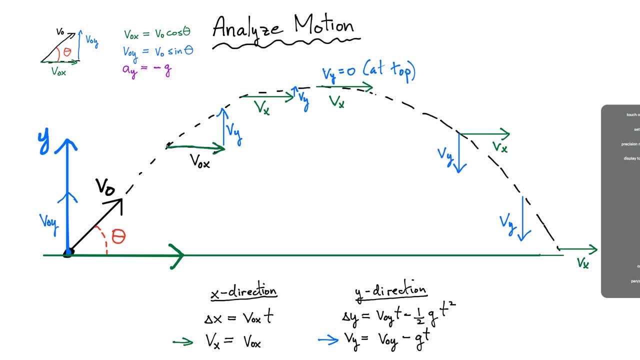 since I know the magnitude, the magnitudes of each component, I can go ahead and plot the vector. Vy is a function of time. Likewise, for this one, I know both components of the vector. I can go ahead and plot the velocity vector. 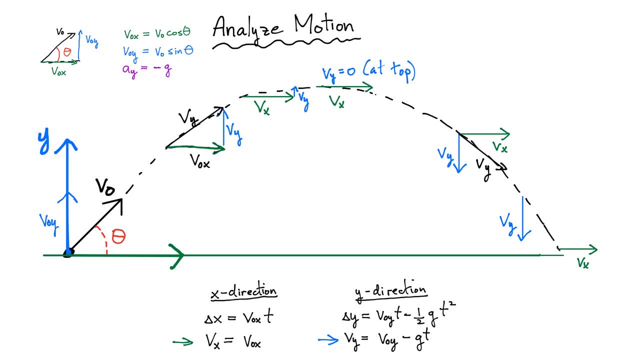 Right before it hits the ground. again, you're going to have a component in the Y direction and you can go ahead and plot the total component of the velocity or the total velocity which is going to be at some angle. Now it turns out. 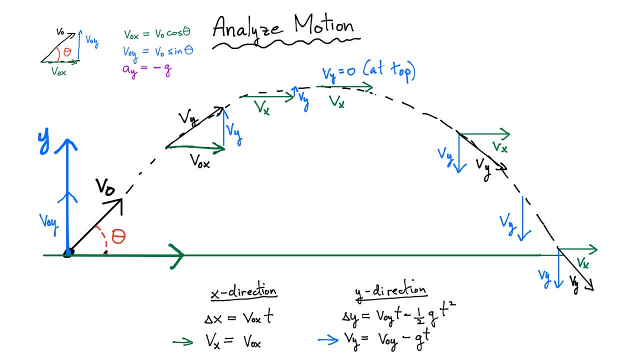 that if you've launched this projectile at an angle theta, this picture is actually symmetric with respect to the center. The center we said. the velocity in the Y direction is equal to zero. Actually, what happens now, right before it hits the ground? 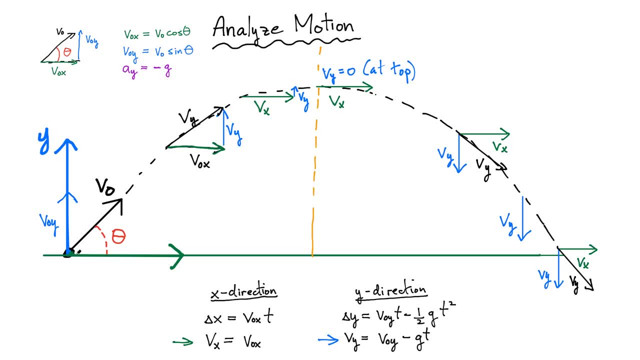 well, the X component of the velocity is simply equal to the initial one. That doesn't change. We know that's the same everywhere. So this vector at the start is equal to the vector at the end, However, the one in the Y component. 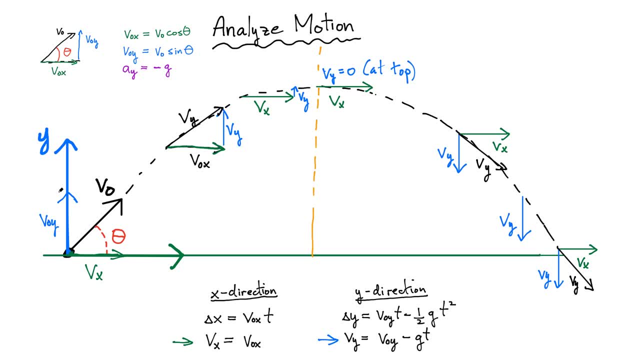 basically simply switches signs. So if I had an initial velocity in the Y direction that was pointing up and had a particular magnitude right before it hits the ground, that vector is going to have the same length as the initial length, except it's going to be in the opposite direction. 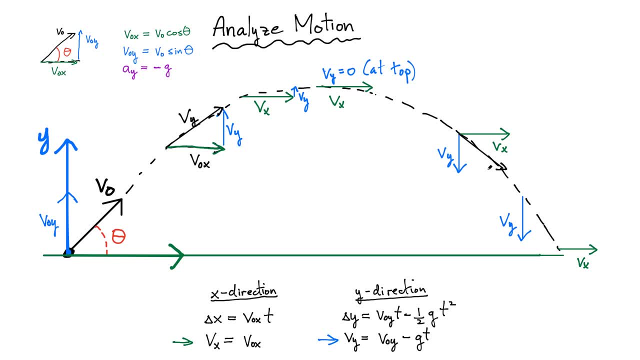 Likewise for this one. I know both components of the vector. I can go ahead and plot the velocity vector Right before it hits the ground. again, you're going to have a component in the y direction and you can go ahead and plot the total component of the velocity, or the total velocity which is going to be at some angle. 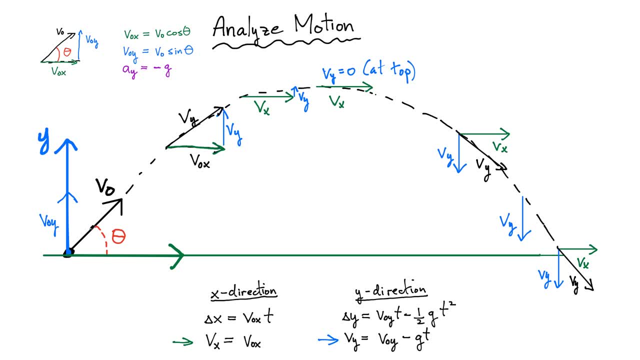 Now it turns out that if you've launched this projectile at an angle theta, this picture is actually symmetrical. It's symmetrical with respect to the center. The center, we said. the velocity in the y direction is equal to zero. Actually, what happens now, right before it hits the ground? well, the x component of the velocity is simply equal to the initial one. 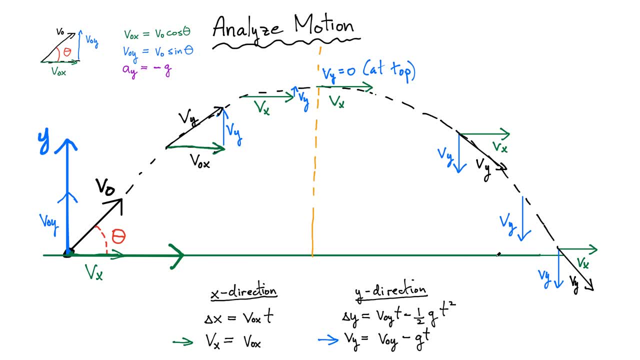 That doesn't change. We know that's the same everywhere. so this vector at the start is equal to the vector at the end. However, the one in the y component basically simply switches signs. So if I had an initial velocity In the y direction that was pointing up and had a particular magnitude right before it hits the ground, that vector is going to have the same length as the initial length, except it's going to be in the opposite direction. 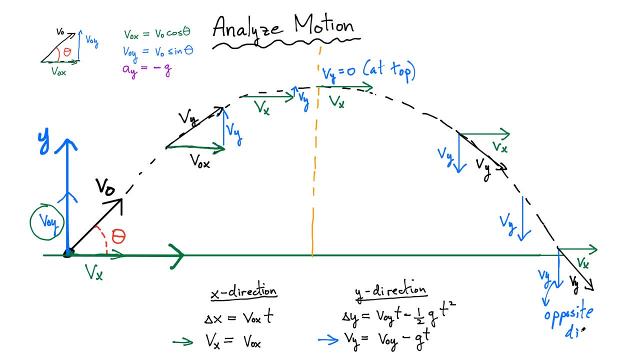 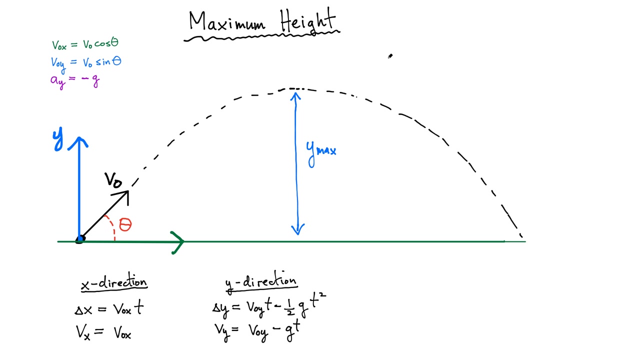 So opposite direction, Okay. so now let's look at things a little bit more quantitatively. We're going to look at the maximum height that the projectile can achieve, And we're also going to look at how far it could travel. Okay, so let's first start by finding the maximum height. 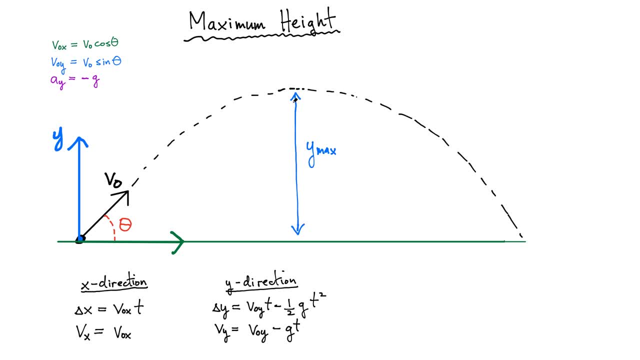 Well, I'm looking for a y displacement and I want to know, when the y displacement is as big as you can get, Where to start. Well, we have an equation down here. This tells me the y displacement, So let's substitute that value there. 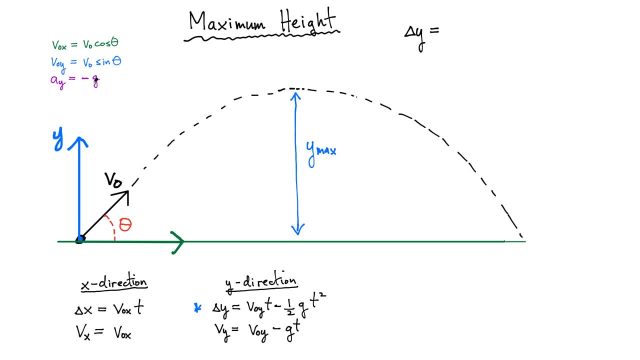 The y displacement is: It's my initial velocity, times time. Let's substitute the value of the initial velocity, That's v-naught sine theta, multiplied by time minus one-half little g times t-squared. This tells me the height at every single time. 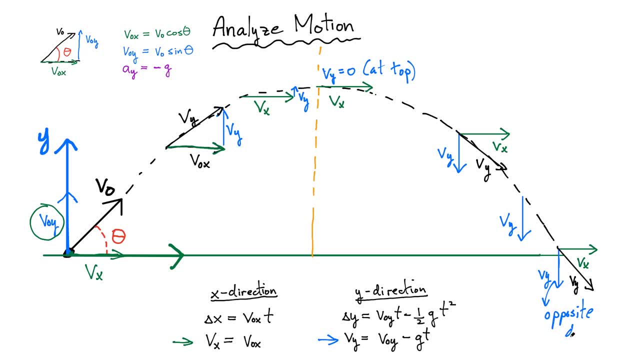 So opposite direction, Okay. so now let's look at things a little bit more quantitatively. We're going to look at the maximum height that the projectile can achieve, and we're also going to look at how far it could travel. Okay, so let's first start. 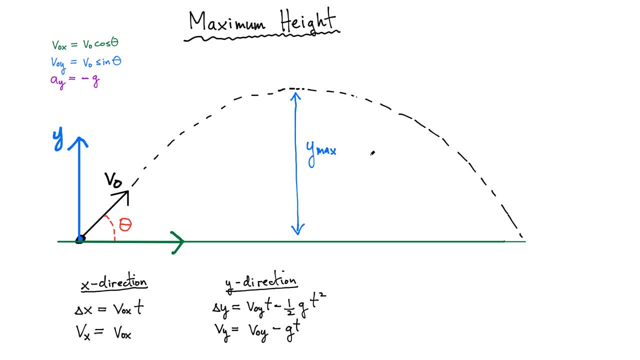 by finding the maximum height. Well, I'm looking for a Y displacement and I want to know, when the Y displacement is as big as you can get, Where to start. Well, we have an equation down here. This tells me the Y displacement. 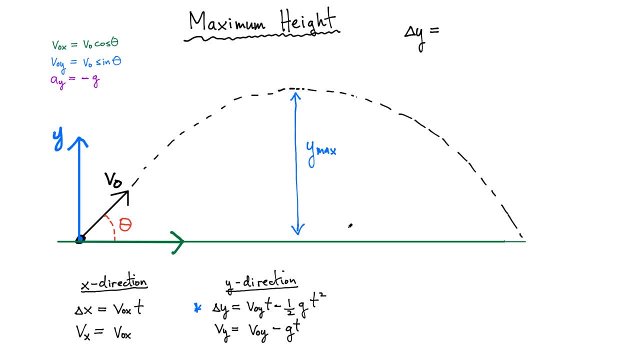 So let's substitute that value there. The Y displacement is: it's my initial velocity, times time. Let's substitute the value of the initial velocity. It's V naught sine theta, multiplied by time minus one half little g times t squared. 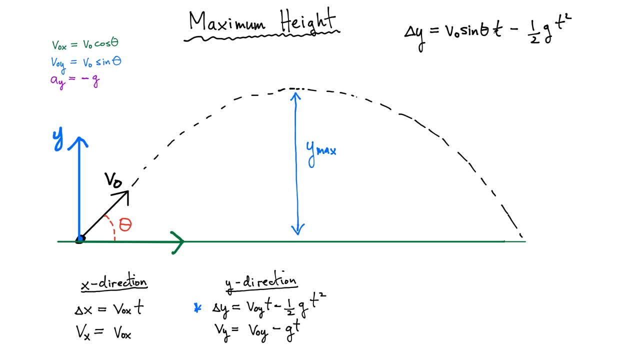 This tells me the height at every single time. If I substitute zero here for time, I get zero. Yeah, that's because I started right here on the ground. So how do I get the maximum velocity? Well, typically, you know the angle. 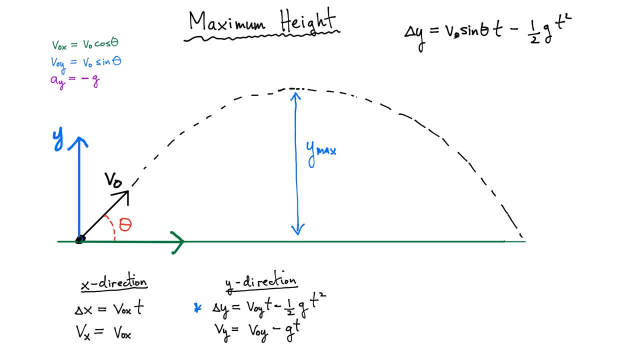 at which you threw the object. You know the initial velocity. You just don't know which time do I substitute into this equation. So for that you have to look at what's going on over here at the top. What else do we know about the top? 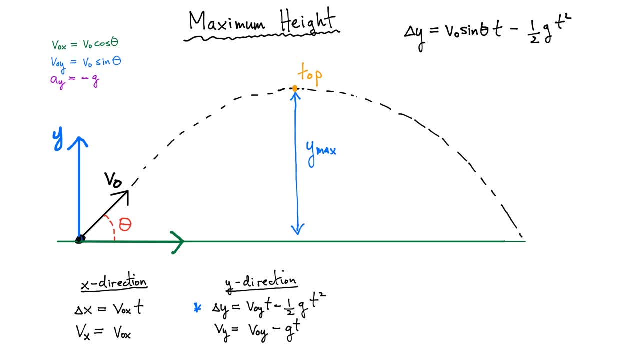 From the previous discussion. I said that at the top you have something very special. that happens That the Y component of the velocity at the top is equal to zero. Well, let's look at our equation now. for the Y velocity, That means that 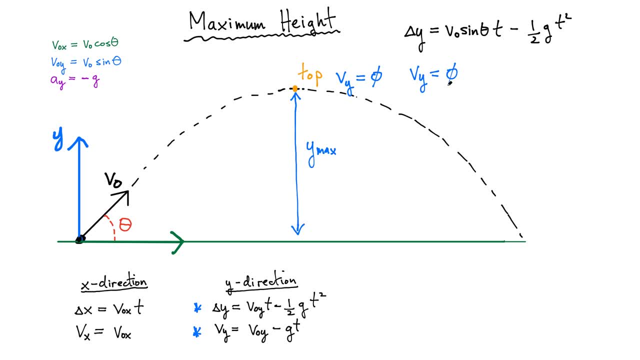 Vy equals to zero. at the top That has to be equal to V, zero sine of theta, minus little g times time. So I have two expressions here. I have one that gives me my displacement and I have another one now that I can use. 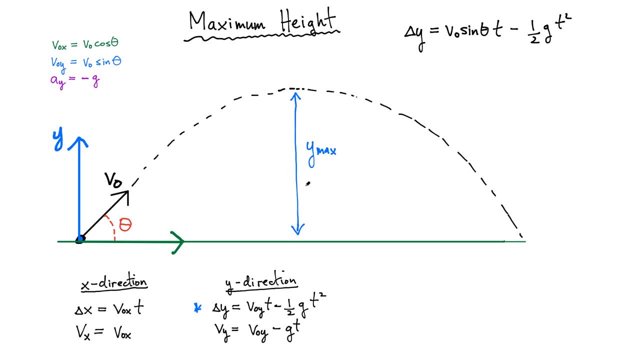 If I substitute zero here for time, I get zero. So yeah, that's because I started right here on the ground. So how do I get that? How do I get the maximum velocity? Well, typically you know the angle at which you threw the object. 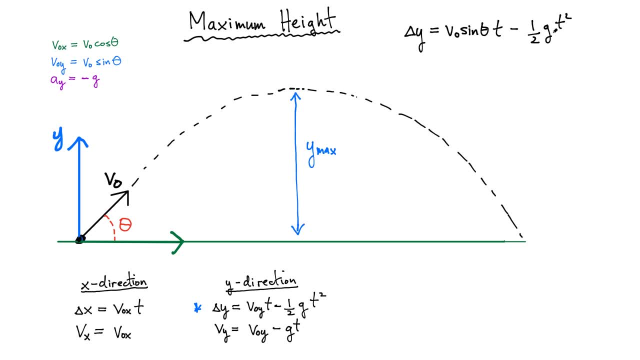 You know the initial velocity. You just don't know which time do I substitute into this equation. So for that you have to look at what's going on over here at the top. What else do we know about the top From the previous discussion I said that at the top you have something very special that happens. 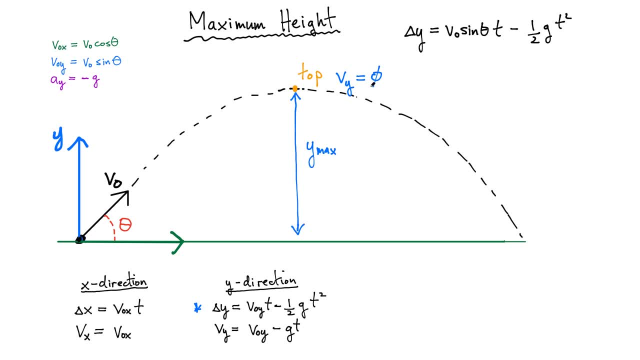 That the y component of the velocity at the top is equal to zero. Well, let's look at our equation now for the y velocity. That means that v-y equals to zero at the top. That has to be equal to v-zero sine of theta minus little g times time. 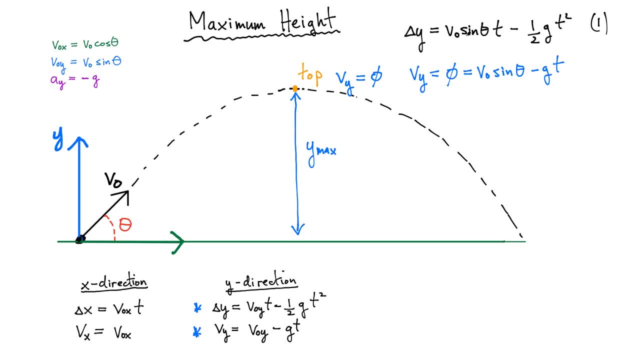 So I have two expressions here. I have one that gives me my displacement and I have another one now that I can use to figure out which time I should actually substitute. I can actually substitute into equation one. So by solving equation two we get the time to go to the top. 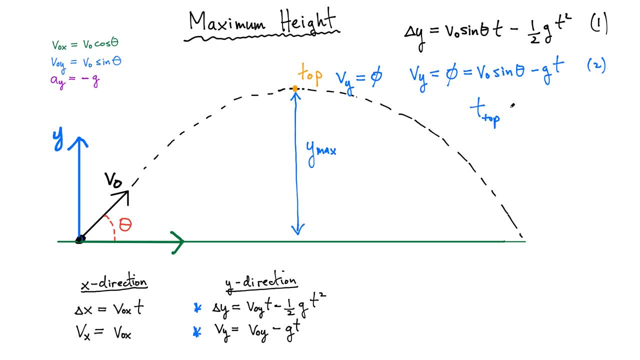 The time to go to the top. now again, I'm just going to isolate for the time and solve this equation. I'm going to get v-zero sine of theta divided by little g. This is how much time it takes for the projectile to go to the top. 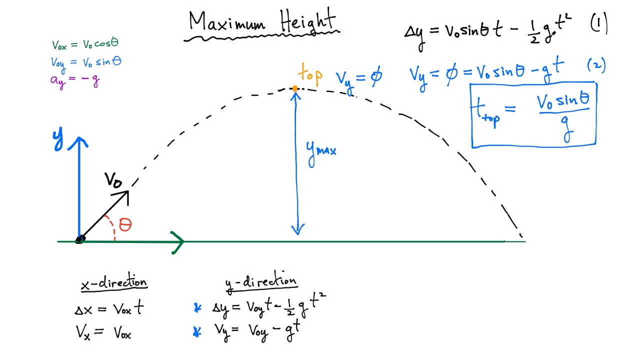 So what can I do with this expression? Well, if you go back now and you substitute this expression into equation one, you're going to get the displacement or the maximum displacement. So delta y max- I guess you'd call it delta y- is going to be equal. 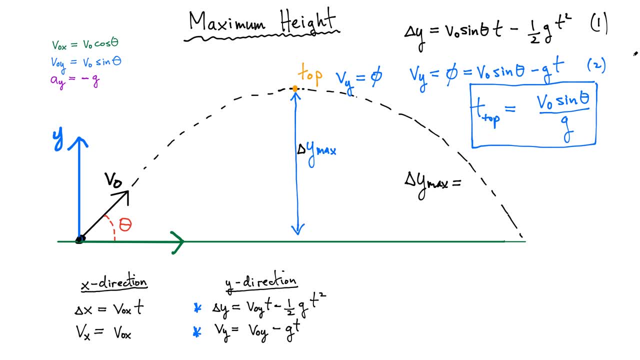 Again, the only unknown in this equation is really that time. So if we substitute everything in, what are we going to get? We have v-not sine theta times time. The time also has a v-not sine theta. The time also has a v-not sine theta. 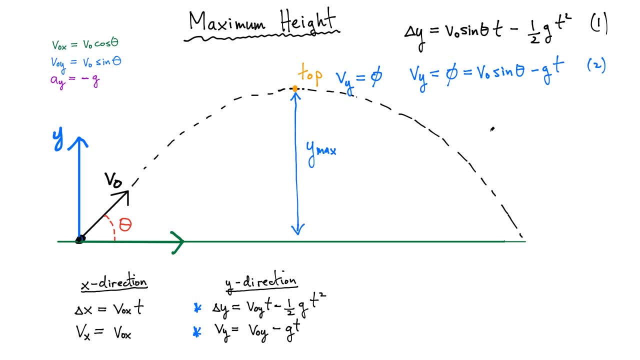 to figure out which time I should actually substitute into equation one. So by solving equation two, we get the time to go to the top. The time to go to the top. now again, I'm just going to isolate for the time and solve this equation. 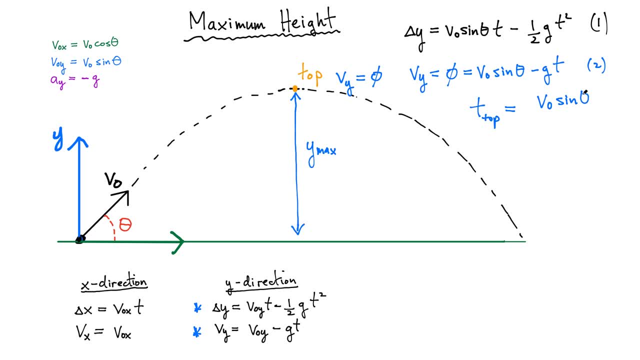 I'm going to get V, zero sine of theta, divided by little g. This is how much time it takes for the projectile to go to the top. Now, what can I do with this expression? Well, if you go back now and you substitute this expression into equation one, 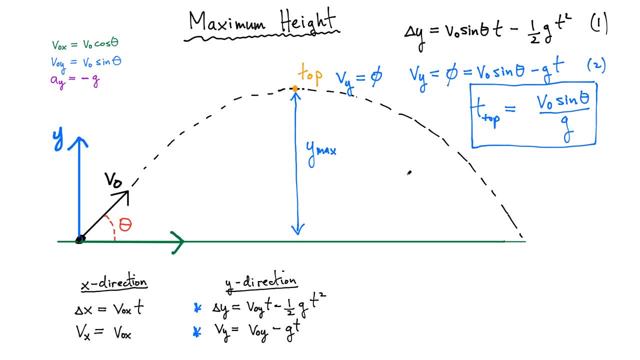 you're going to get the displacement or the maximum displacement. So delta Y max- maybe I should call it delta Y- is going to be equal again. the only unknown in this equation is really that time. So if we substitute everything in 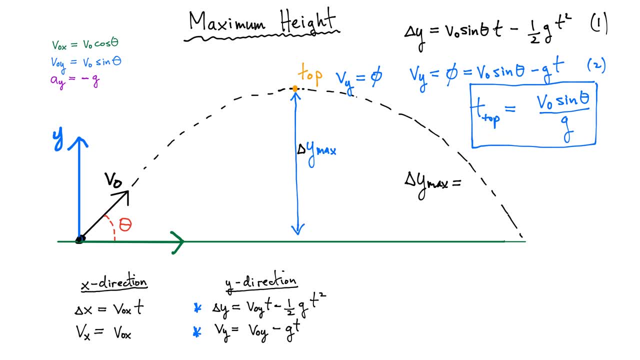 what are we going to get? We have V naught sine theta. times time Time also has a V naught sine theta, So this term here becomes V naught sine theta. all of this is squared divided by little g Minus one half. 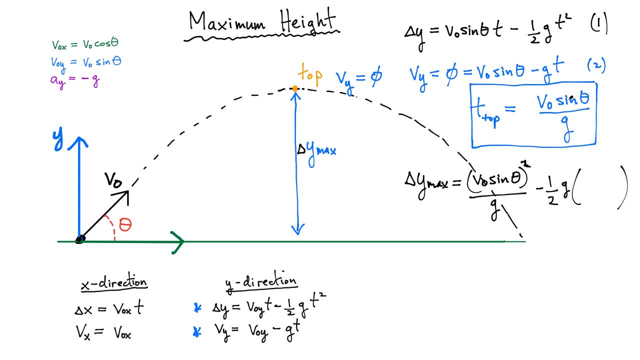 my acceleration is little g, and now what do I have? Well, I've got t squared, which again is this expression over here, Divided by little g. I can't forget to square the whole thing. Now. this looks very complicated. 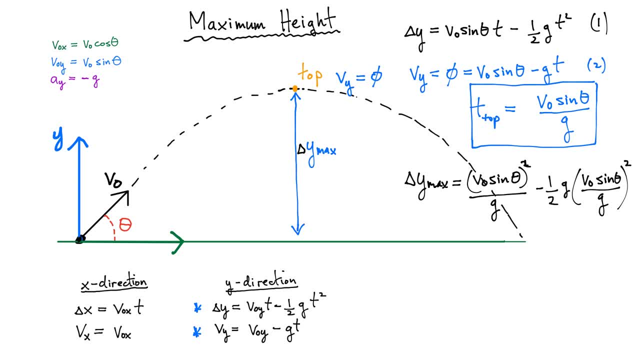 however, the terms look almost identical to each other. If you simplify this, you're going to get that the maximum displacement or the maximum height that you're going to achieve is going to be V. naught sine theta, this term remains squared. sine theta will remain squared. 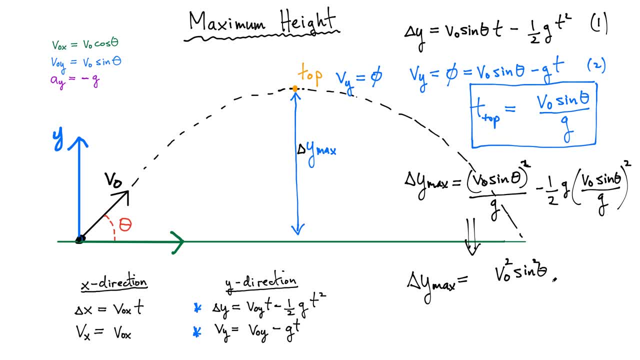 you're going to have one in the front minus a half, so you're going to be left with two times little g. So here's my expression now for the maximum height that my projectile is going to reach. So one thing you see is, when is this height the maximum? 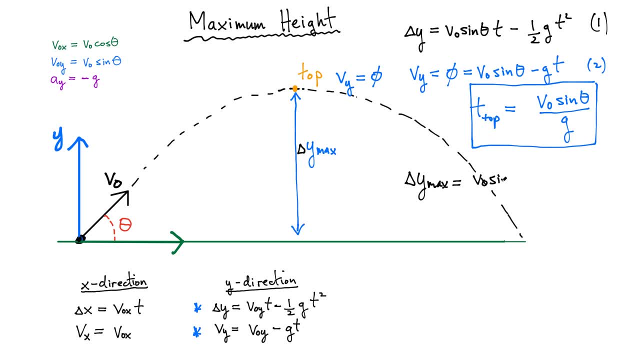 So this term here becomes v-not sine theta. All of this is squared, divided by little g Minus one half. my acceleration is little g. and now what do I have? Well, I've got t squared, which is again: is this expression over here? 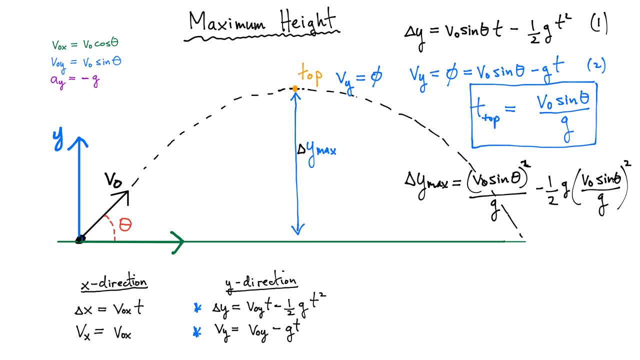 Divided by little g, and I can't forget to square the whole thing Now. this looks very complicated. However, the terms look almost identical to each other. If you simplify this, you're going to get that- the maximum displacement or the maximum height that you're going to achieve. 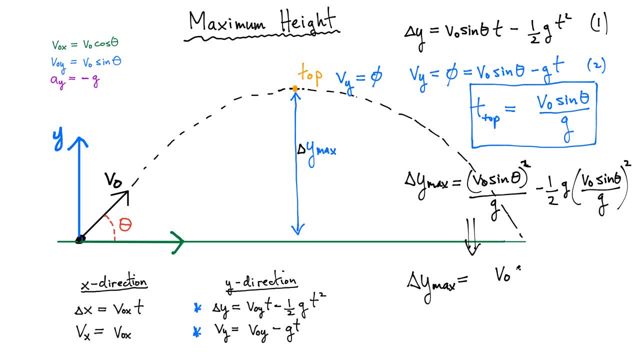 is going to be v-not sine theta. This term remains squared. Sine theta will remain squared. You're going to have one in the front minus a half, and you're going to be left with two times little g. So here's my expression. now for the maximum height that my projectile is going to reach. 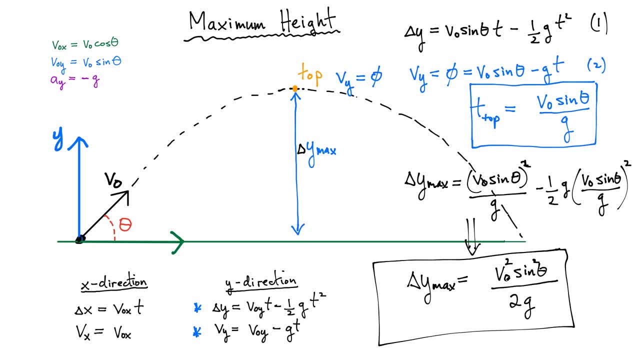 So one thing, you see is, when is this height the maximum For any given velocity? how do I get the biggest vertical displacement? I'm going to get the biggest vertical displacement whenever sine of the angle theta is equal to one. And when do I get sine theta equal to one? 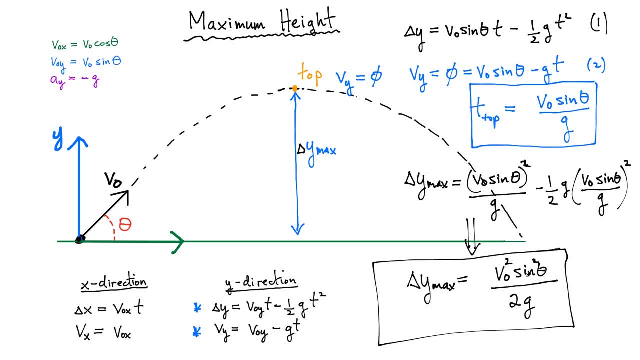 That's when the angle theta equals to 90. That's if I shoot the object straight up. that's when I'm going to get the highest maximum height. Okay, and the last thing I want to look at today is the range of the projectile. 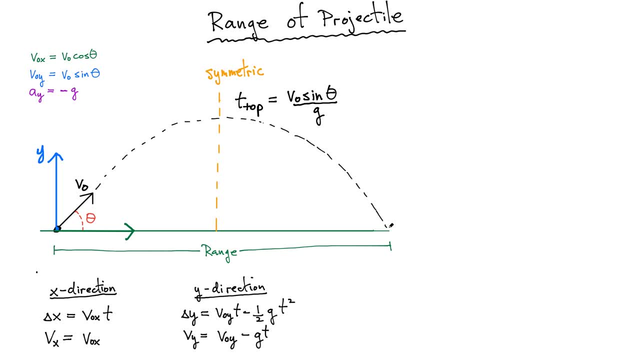 And that's basically how far is the projectile going to travel? What's the horizontal displacement of this projectile? Well, if I want to know the horizontal displacement of the projectile, I should use an equation that describes the horizontal displacement. So, in this case, I'm going to want to know my horizontal displacement x. 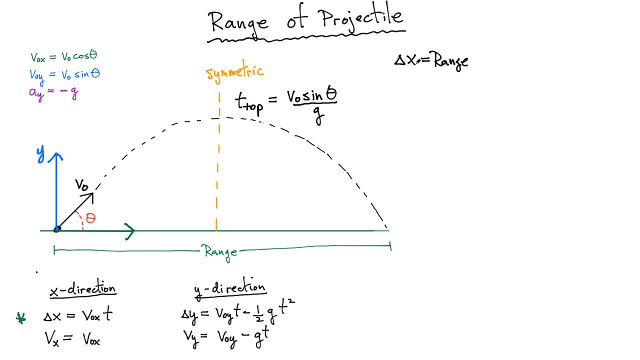 which is what I'm going to call my range, because I want to find what the maximum displacement in the x direction is. That's what I've defined by the green line here. That is simply going to be equal to my initial velocity in the x direction. 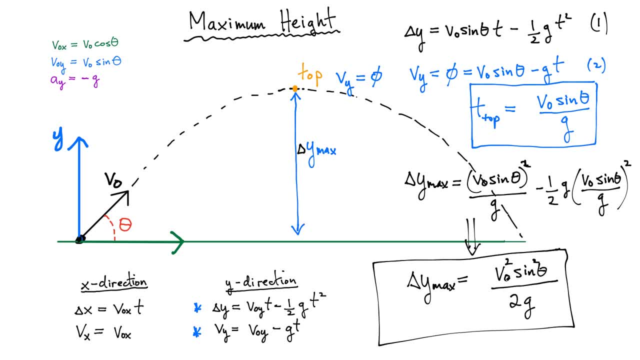 For any given velocity. how do I get the biggest vertical displacement? I'm going to get the biggest vertical displacement whenever sine of the angle theta is equal to one. And when do I get sine theta equal to one? That's when the angle theta equals to 90.. 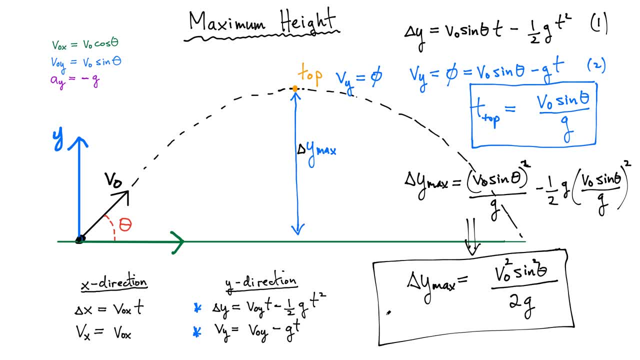 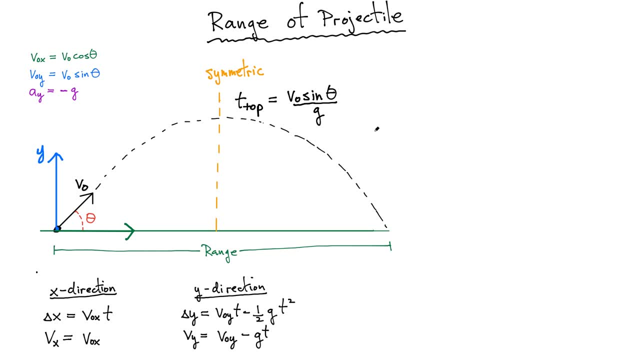 That's if I shoot the object straight up. that's when I'm going to get the highest maximum height. Okay, and the last thing I want to look at today is the range of the projectile, And that's basically how far is the projectile going to travel? 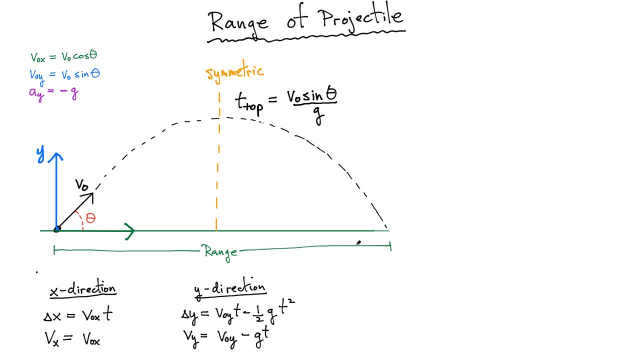 What's the horizontal displacement of this projectile? Well, if I want to know the horizontal displacement of the projectile, I should use an equation that describes the horizontal displacement. So, in this case, I'm going to want to know my horizontal displacement x. 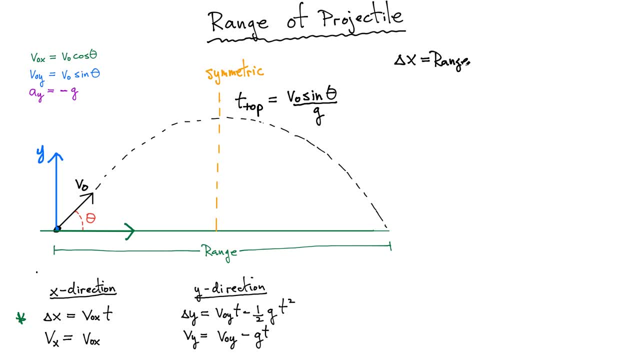 which is what I'm going to call my range, because I want to find what the maximum displacement in the x direction is. That's what I've defined by the green line here. That is simply going to be equal to my initial velocity in the x direction. 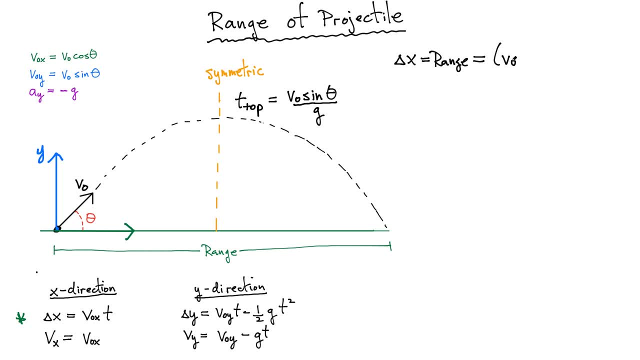 which I know. it's simply v, zero, cos of theta multiplied by the time. So if I know an expression, if I know an expression for the time, I could substitute it into this equation. let's call it equation one, and I can find what the range of the projectile is. 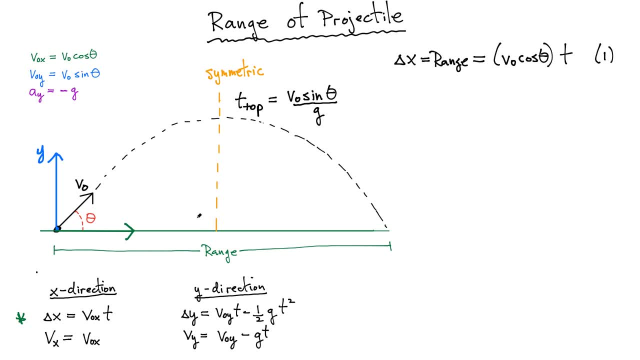 So there's one more thing that I want to mention again that's very important about projectile motion is that everything is symmetric. about the top, For example, if you know the time it takes to get to the top, which we just calculated in the previous example, 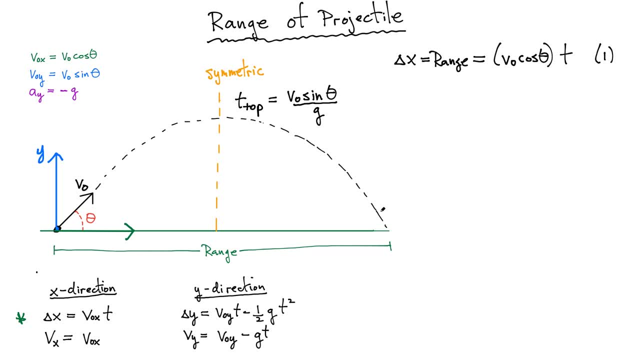 that means that the total flight time is going to be: the total time that the particle is in the air is simply going to be twice the value it takes to get to the top. Let me write it down here: Two times t top. So the total time, the total flight time here. 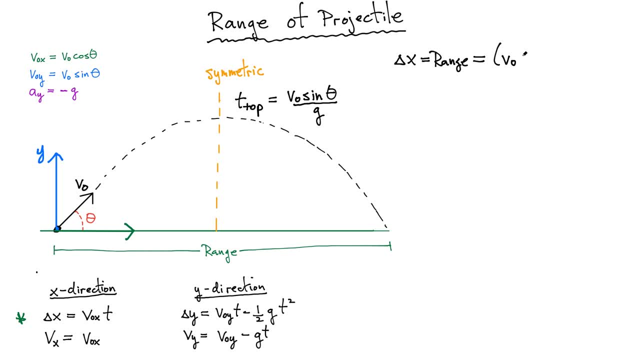 which I know. It's simply v, zero, cos of theta multiplied by the time. So if I know an expression for the time, I could substitute it into this equation. let's call it equation one, and I can find what the range of the projectile is. 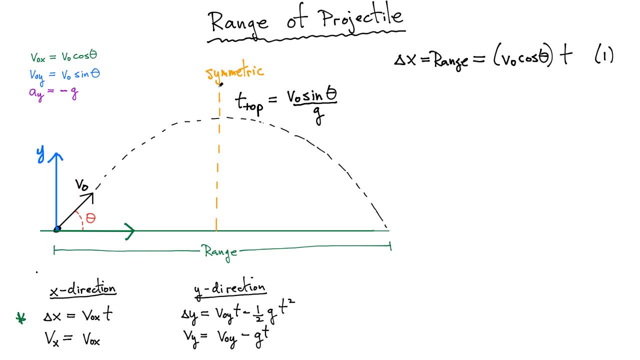 So there's one more thing that I want to mention again that's very important about projectile motion is that everything is symmetric. about the top, For example, if you know the time it takes to get to the top, which we just calculated in the previous example, 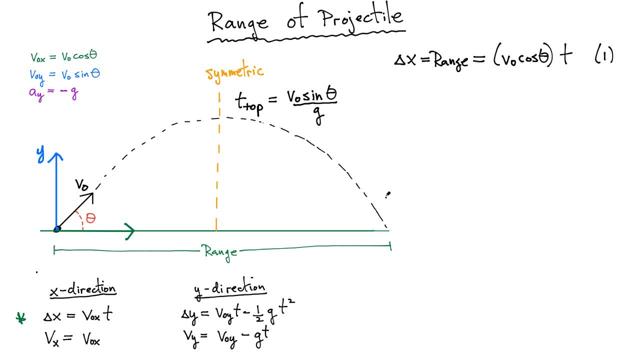 that means that the total flight time, the total time that the particle is in the air, is simply going to be twice the value it takes to get to the top. Let me write it down here: Two times t top. So the total time, the total flight time here. 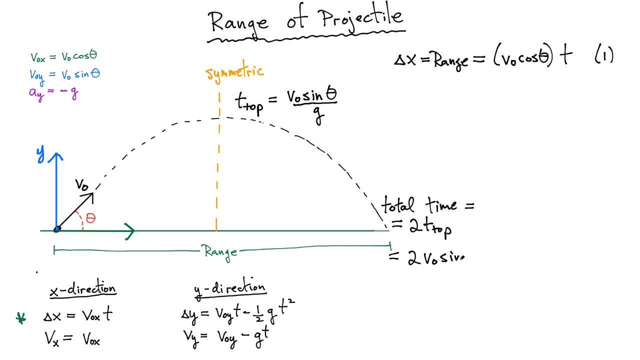 is going to be times v zero sine of theta divided by little g. That's my total time, So that's really the only expression that I'm missing. So if I go back now, I can write that the range is simply going to be equal to v zero cos of theta. 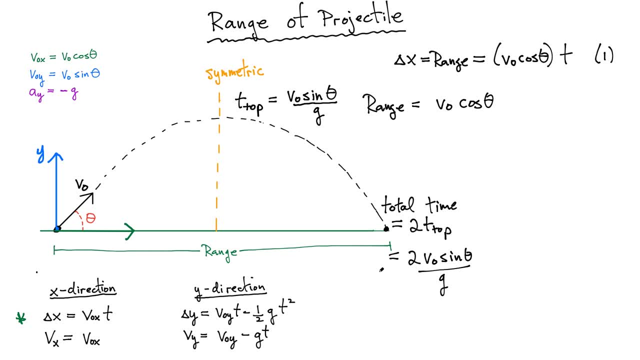 and I want to know the time. Well, I need to know the time right at this position, right before it hits the ground. That's the total flight time. So that's simply two times v, zero sine of theta divided by little g. 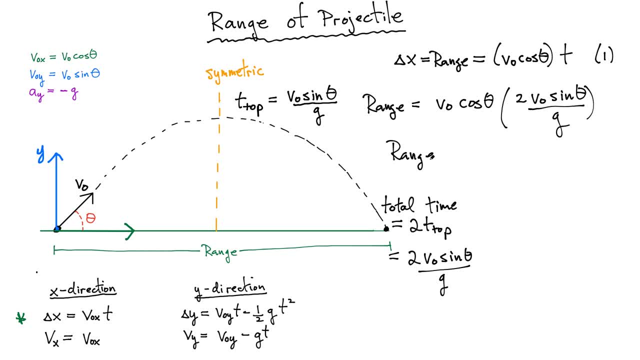 If you simplify everything, our final expression for the range, that's our maximum x displacement, is going to be two v zero squared sine theta, cos theta divided by little g. And there you have it, folks. So this is the expression that we have for the range. 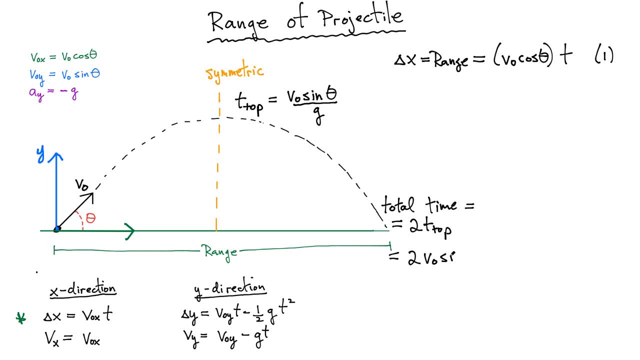 is going to be two times v zero sine of theta divided by little g. That's my total time, So that's really the only expression that I'm missing. So if I go back now, I can write that the range is simply going to be equal to v zero cos of theta. 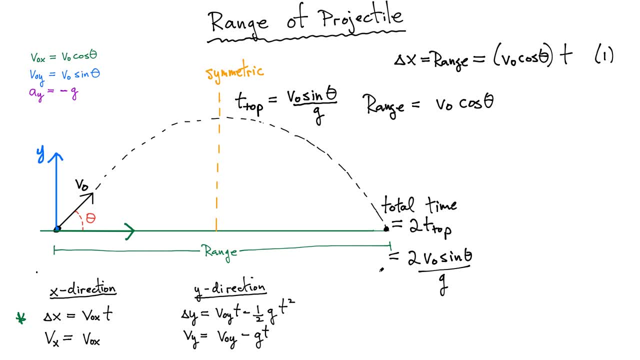 and I want to know the time. Well, I need to know the time right at this position, right before it hits the ground. That's the total flight time. So that's simply two times v, zero sine of theta divided by little g. 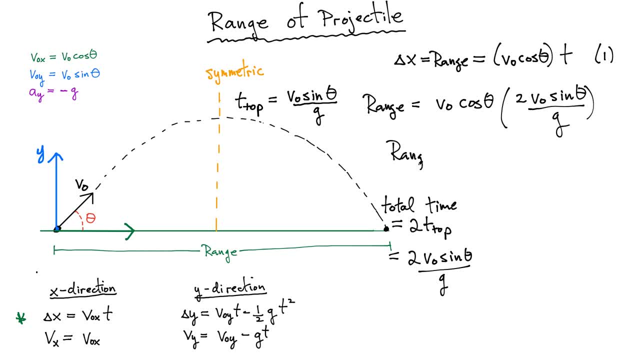 If you simplify everything, our final expression for the range, that's our maximum x displacement, is going to be two v zero squared sine theta, cos theta divided by little g. And there you have it, folks. So this is the expression that we have for the range. 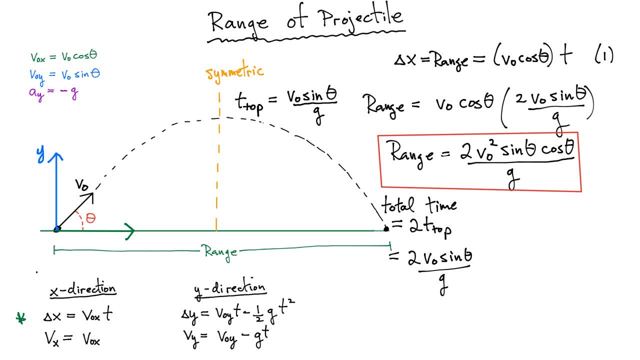 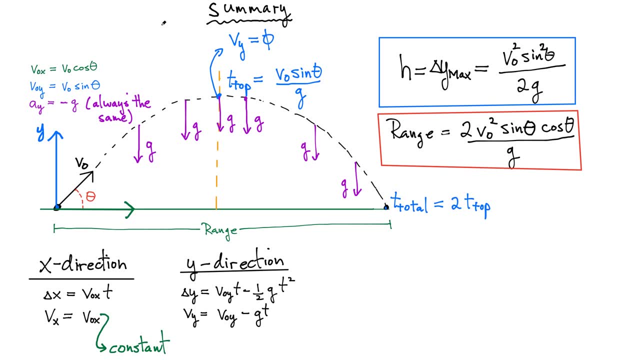 of our projectile. Okay, to summarize everything we've learned today, we've broken down our initial velocity into x and y components. Remember: the acceleration is only in the y direction. There's no acceleration in the x direction and the acceleration in the y direction is the same everywhere. 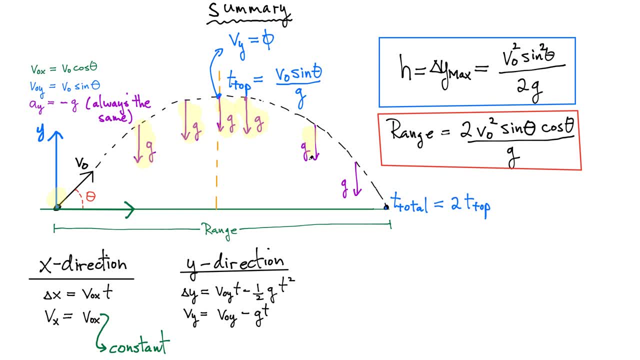 It's the same here, same there. Regardless of where you draw that vector, you have to have the same length in the same direction. To analyze the motion in the x direction, we looked at the x displacement and the velocity in the x direction. 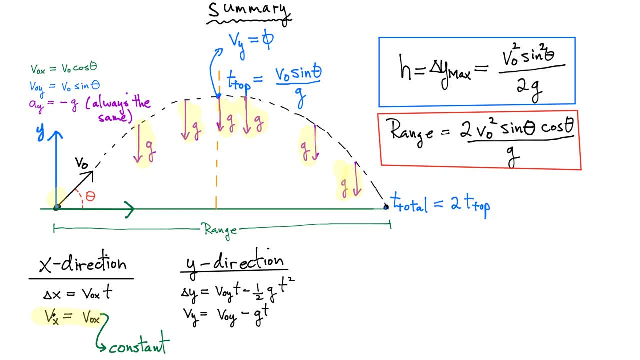 The velocity in the x direction is very easy. It's constant, It doesn't change because there's no acceleration in the x direction. Therefore, the displacement in the x direction takes on a very, very simple form. It's simply my initial velocity multiplied by the time. 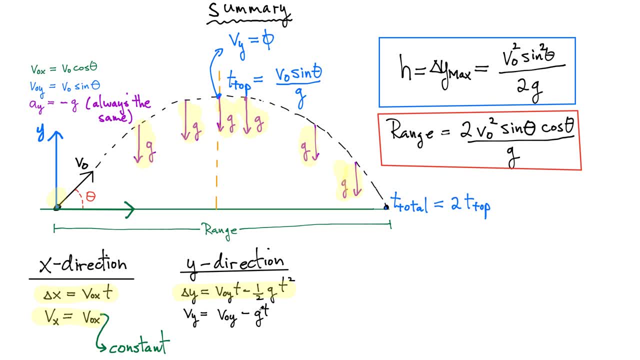 In the y direction things are a little bit more complicated because I have to include the acceleration terms And here are the expressions for the displacement and the velocity. We also looked at the top. The top's a very special point for projectile motion because the velocity in the y direction goes to zero at the top. 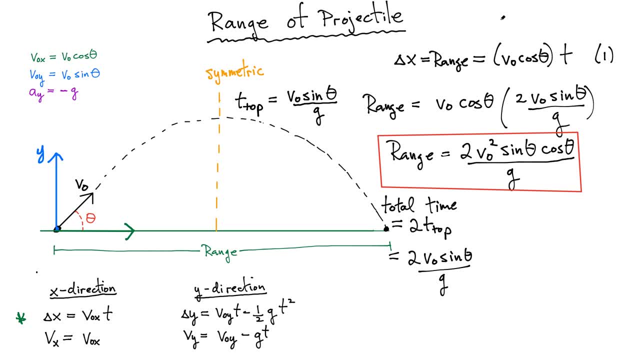 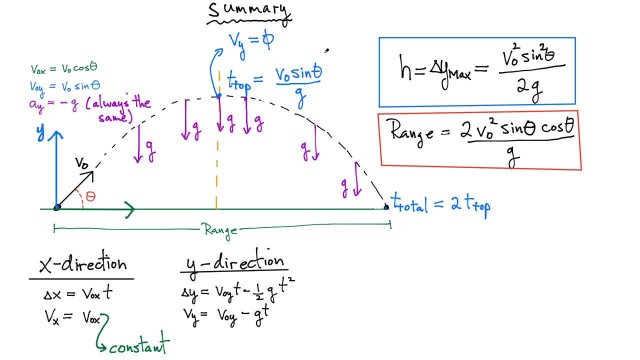 of our projectile. Okay, to summarize everything we've learned today, we've broken down our initial velocity into x and y components. Remember: the acceleration is only in the y direction. There's no acceleration in the x direction and the acceleration in the y direction. 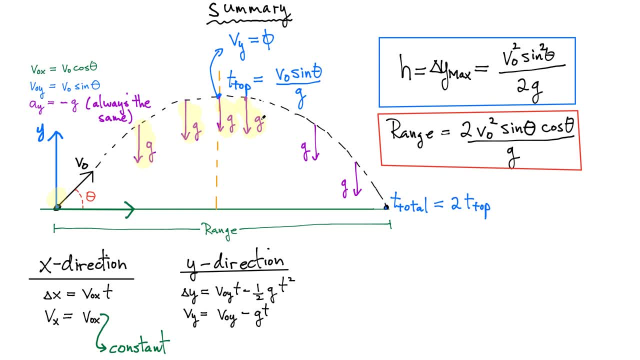 is the same everywhere. It's the same here, same there. Regardless of where you draw that vector, you have to have the same length in the same direction. To analyze the motion in the x direction, we looked at the x displacement and the velocity in the x direction. 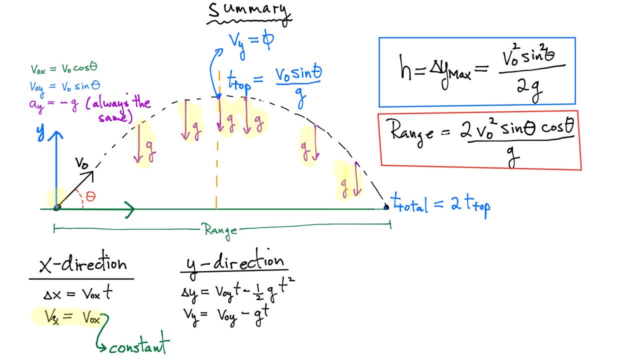 The velocity in the x direction is very easy. It's constant, It doesn't change because there's no acceleration in the x direction. Therefore, the displacement in the x direction takes on a very, very simple form. It's simply my initial velocity. 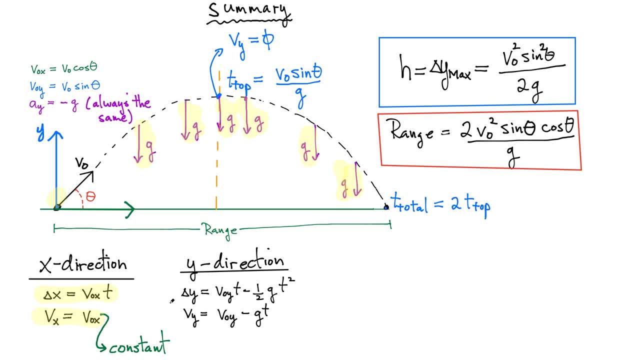 multiplied by the time. In the y direction things are a little bit more complicated because I have to include the acceleration terms, And here are the expressions for the displacement and the velocity. We also looked at the top. The top's a very special point for projectile motion. 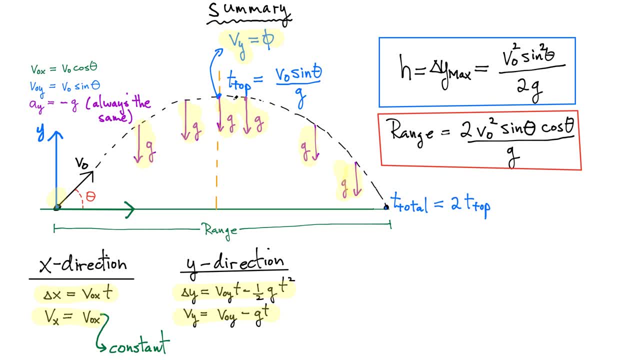 because the velocity in the y direction goes to zero at the top, And if you solve the expression, you obtain that the amount of time it takes to go to the top is simply v, zero sine theta, divided by little g. And since everything is symmetric, about the middle. 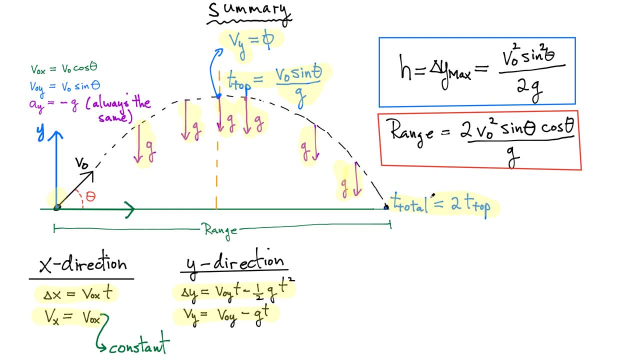 that means it's very easy to calculate how much time it takes for the projectile to do the complete trip. It's simply two times or twice as big as the time it takes to go to the top. Using both of these times, we're then able to find what the maximum displacement. 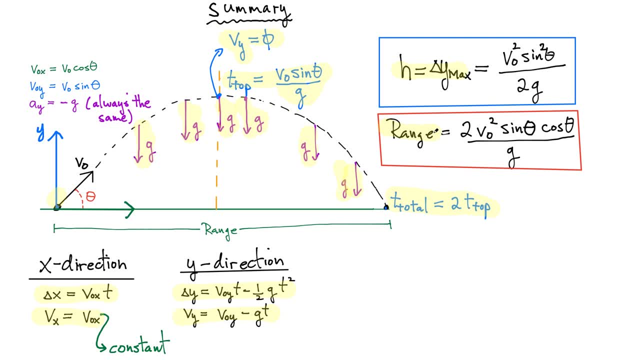 in the y direction is, And we're also able to find what is the maximum range that this projectile will travel. Okay, If you have any questions, folks, just send me an email or leave a comment at the bottom of the video, And also please subscribe to my channel. Thank you.